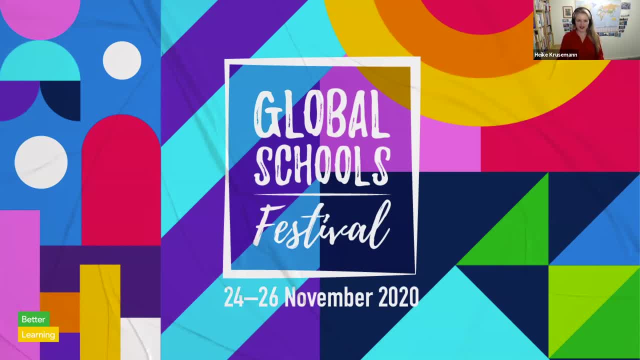 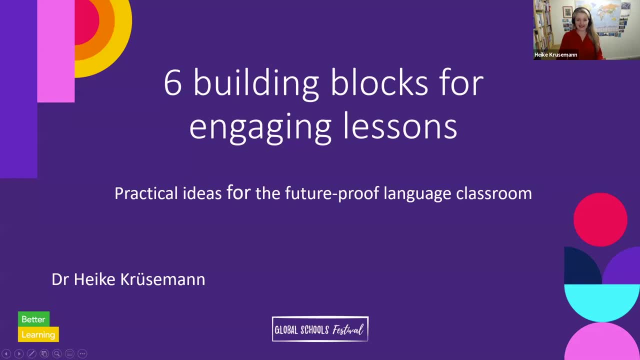 And from all over the world. it's really wonderful to connect with so many of you from all over the world, So thank you so much for joining my talk. Six Building Blocks for Engaging Lessons And, in the current situation, when for many of us the future seems more uncertain than ever before, engaging 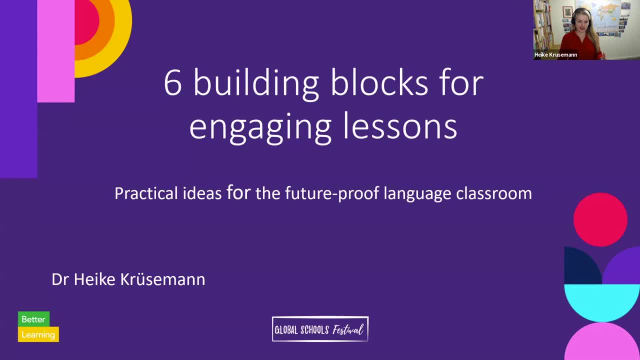 our learners is very much a concern. that's on every teacher's mind, But learners as well. there was a concern. So here at Cambridge we ran a survey where we asked language learners how they felt about the current conditions and looking to the future And they said: 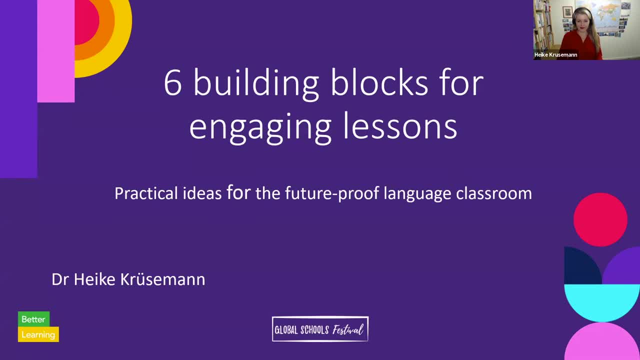 they were struggling to some extent. However, they also told us something very interesting about specific areas where their engagement levels actually received a boost during the current situation, And it's these insights, as well as some academic research, which underpins the ideas that I'm going to share with you today. 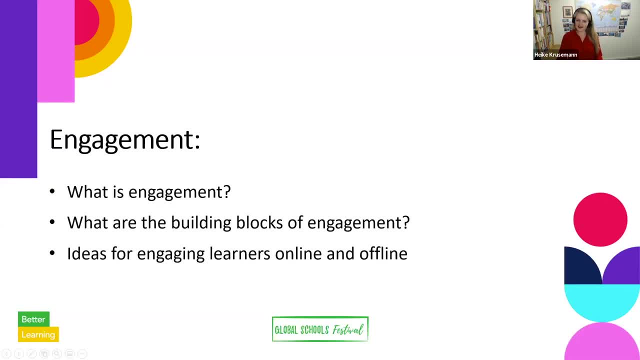 So today we're going to look at the questions: what is engagement, What are the building blocks of engagement? And then we're going to share some ideas of what you can do in your own teaching to engage your learners. So let's get started. Okay, so let's start. 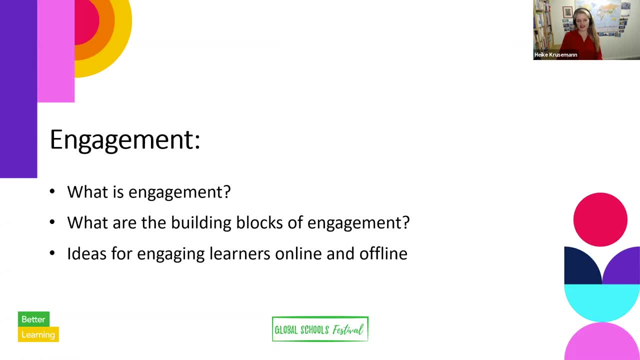 So we're going to start with this one. This question came into my chat box. We'll start with the questions and the answers to the questions. So we've got one first question that just popped in the chat box. It's super easy. So the first question is: how do you? 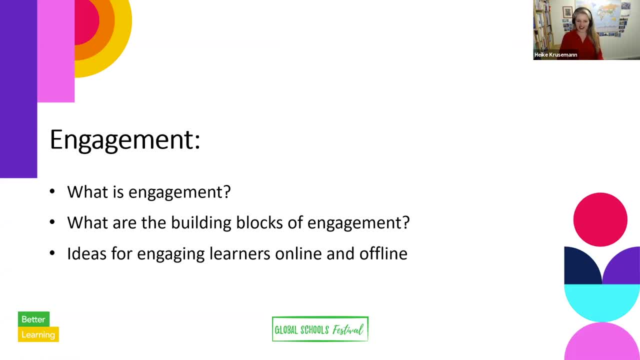 engage your learners And during my talk. you're very, very welcome indeed to type into the chat box during the talk, And this is an opportunity for us all to connect and for you to share your thoughts with me and with other people here as well. And so to start, with now. I have a little fun challenge for you, And that challenge is that near the end of the session I will ask you to type in the chat box a few things that you have learned about me during the talk. So every now and then during the session, I will drop in a little. 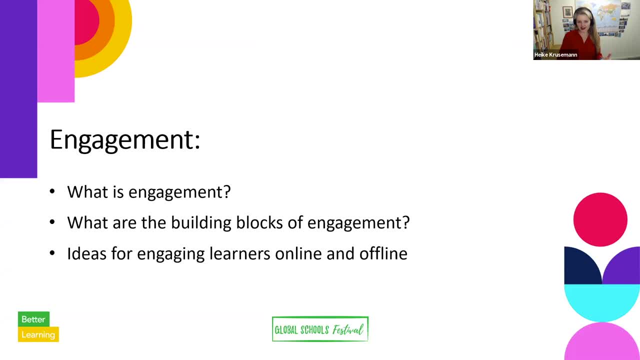 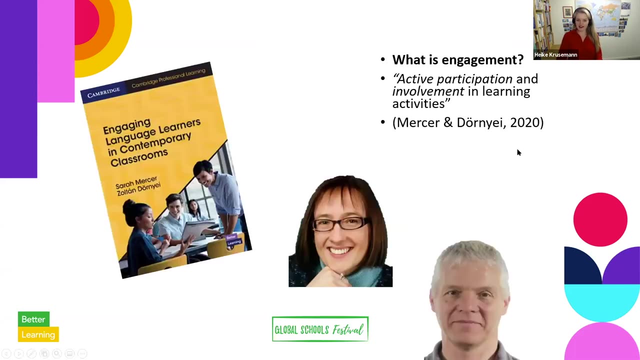 snippet of the fact about me. so an invitation to you now to keep an ear out for that. Okay, so what is engagement? Right? the definition of engagement that I'm going with today is from a book that has come out this year by professors Sarah Mercer and Zoltan Juniaj, and they're both. 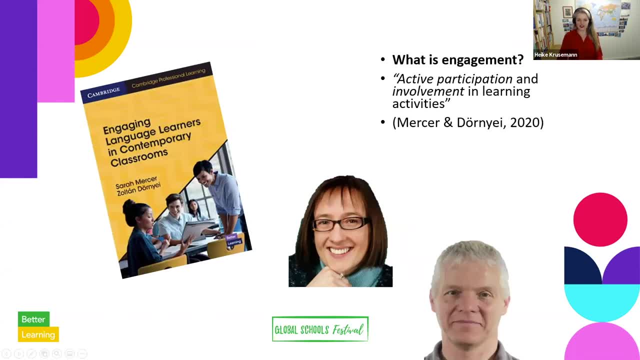 very highly respected researchers in the field of language learning, motivation and engagement, and the book is called Engaging Language Learners in Contemporary Classroom, and I have listed the full reference of this book and of any other books that I will mention during the talk. 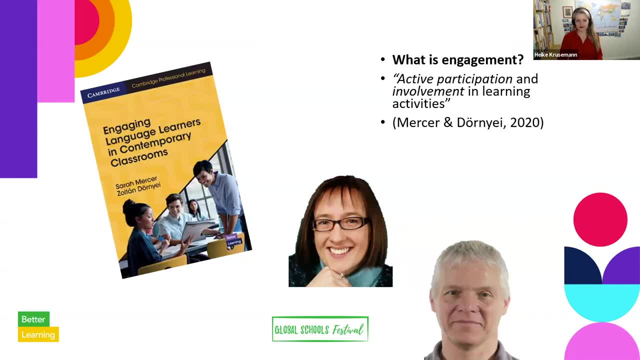 on my last slide, so there is no need for you to take any notes right now. I've got my own copy here and you can see that it is very, very well used, and I just really wanted to share this publication with you because I'm finding it very helpful and also because the 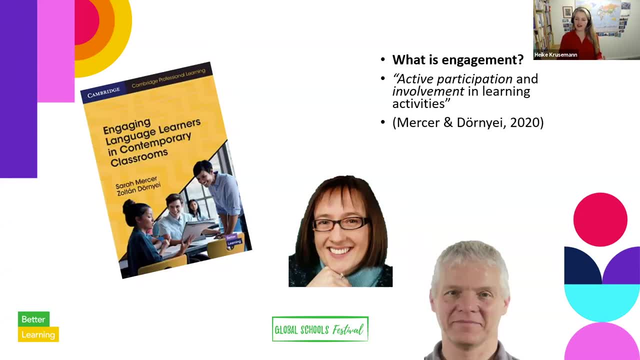 research and the ideas that I'm talking about today are very much aligned with its focus of looking at research on engagement in terms of what's actually helpful for teachers in practical learning. So I'm going to start with the first one and then I'm going to start with the second one. 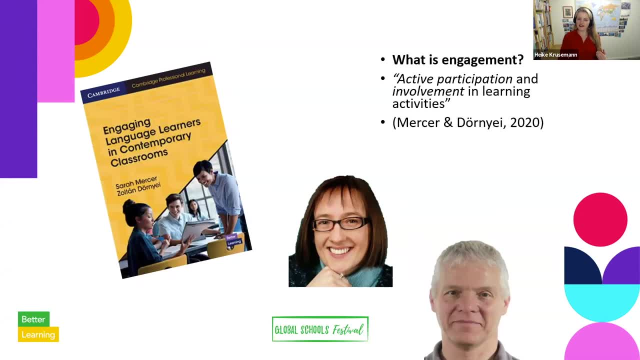 and then I'm going to start with the third one, and then I'm going to start with the fourth one, and then I'm going to start with the fifth one, and then I'm going to start with the sixth one. So Sarah Mercer and Zoltan Dunier define engagement as active participation and 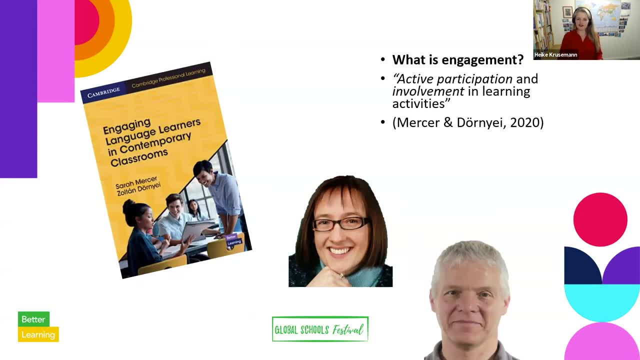 involvement in learning activities. So often people ask what is the difference between engagement and motivation, and the key difference is that you can be as motivated as you like. maybe you have some very important overarching reasons for learning English, but if you're not actively participating and engaging in the learning process, then you 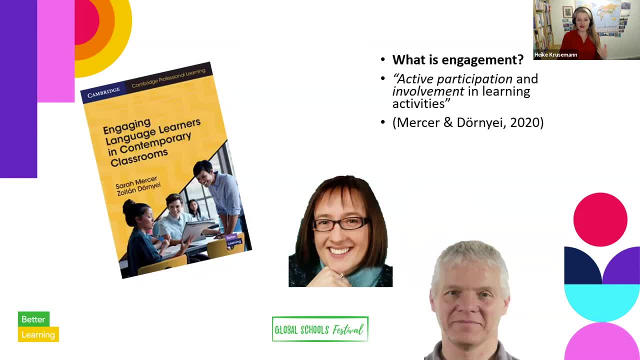 are not learning anything. So often. when we're talking about motivating learners, what we really mean is engaging learners in the learning task and in the face of many distractions coming their way, especially in the form of mobile phones, and these things are all designed to hijack our attention. 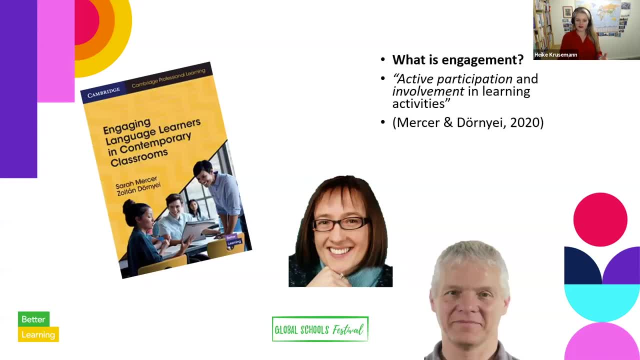 and certainly in my own teaching- and I've taught all age groups, but mainly teenagers and adults, and I've certainly experienced students getting very distracted by mobile phones and maybe you can share in the chat whether you've also experienced this too, just by typing the word yes, if you've also experienced your students getting very. 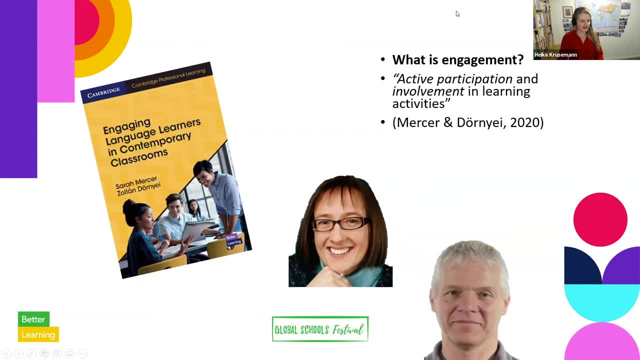 distracted by mobile phones. Okay, I'm trying to get visible that I can see the chat, because I suspect that you're typing away, but I can't see any of that. Okay, sorry. Okay, yes, I can see the chat now. 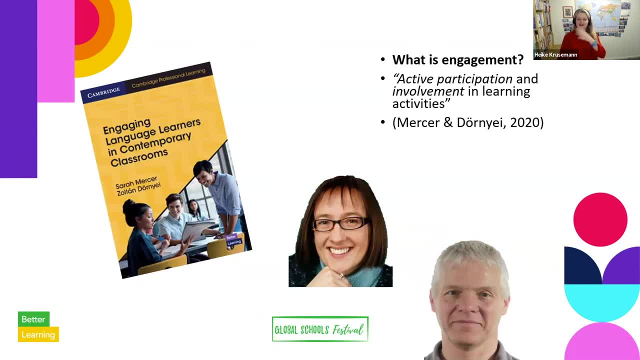 Okay, so that's sorted. Yes, and, as I expected, there is a sea of yeses washing over me. so, definitely, this is something that we've all experienced, so you know what I'm talking about when I mention that. So, but it's probably also fair to say that our students don't really want. 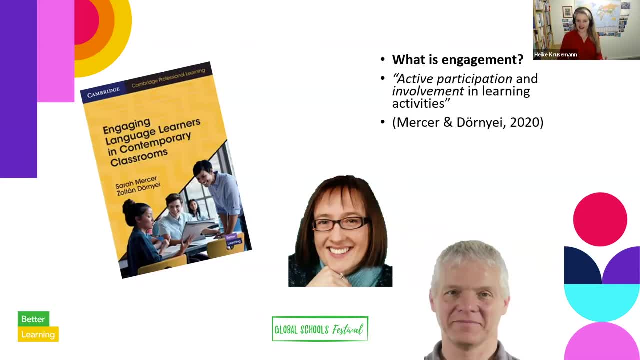 to give in to these distractions. Often, they just don't know how to escape from the magic pull of these marvels of technology that we've all experienced, So I think it's important to that we've all got around us at the moment, And this is exactly where you, as a teacher, can come. 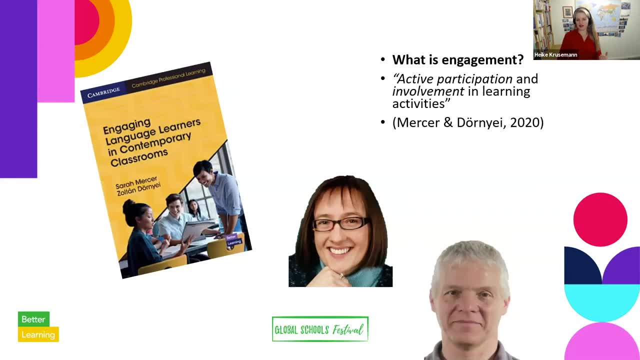 in to help them and to help them focus and to help them engage on the task. So how do you do that Right? so here at Cambridge, we've identified some key factors that we know from research are the six building blocks of language learner engagement, And I would like to go through these. 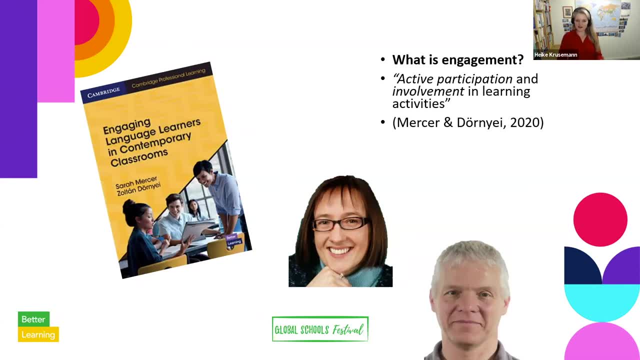 building blocks now, with you and together, we will look at some selected research insights for each one and then we're going to suggest some activity for the class or the course. and we're going to look at some selected research insights for each one And then we're going to suggest some activity. 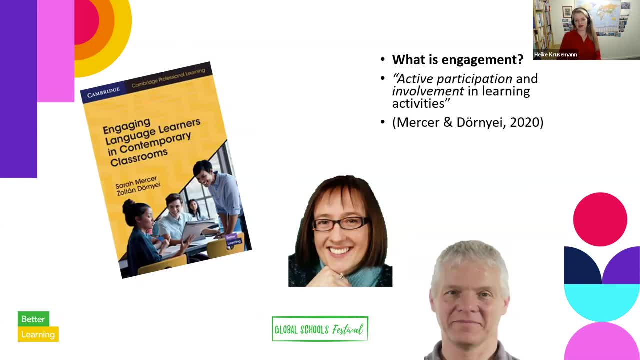 some activities and some action points which you then can implement in your own teaching Right. so think about a situation that many of us are facing right now- and this is certainly the case in the UK, where I live- that you can't really be sure of the classroom conditions which you're. 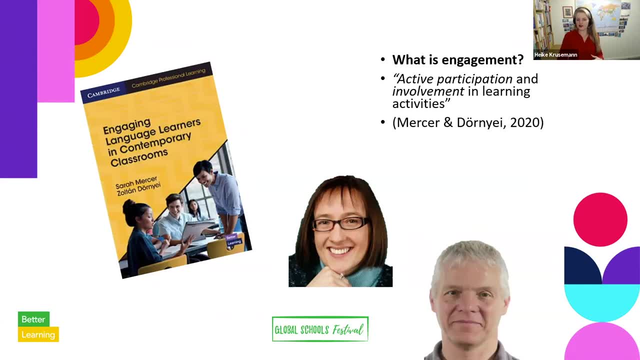 going to face on a day-to-day basis, So you don't know who's going to be there face-to-face, who will be joining online. Sometimes maybe you planned a lesson face-to-face, but then you have to move online with virtually no notice at all and you just don't really know about your student's. 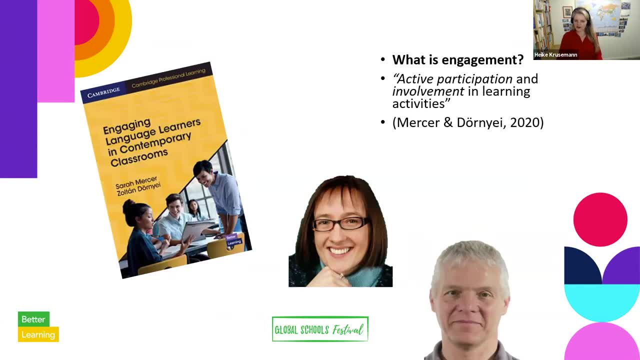 situation either. So maybe you expect that some of them will have done the work that you said. some of them will have made good progress. some of them will have done none of the work and made no progress at all. So you're very aware, whatever situation that you're in, there's going to be lots. 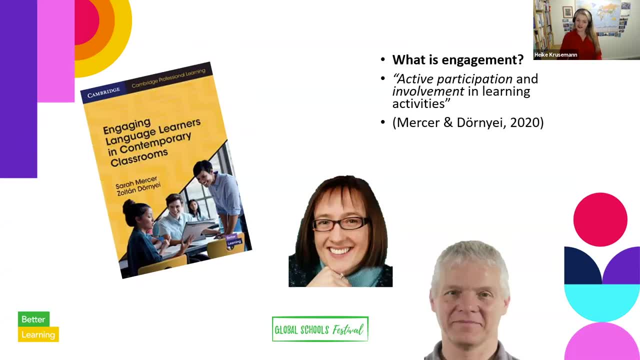 and lots of work to get on with. There is massive pressure on us now to get things done to catch up on missed work, lots of missed work to cover new work. So it's Monday morning, you breeze into your classroom and you say: 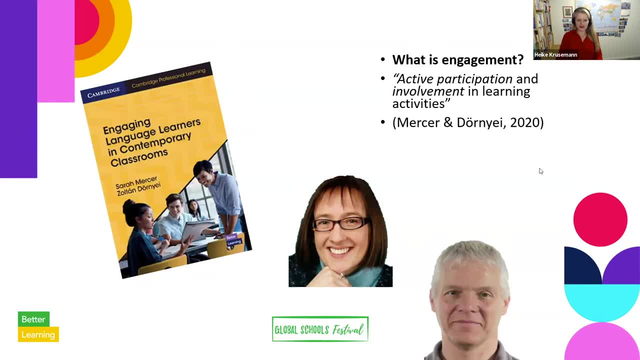 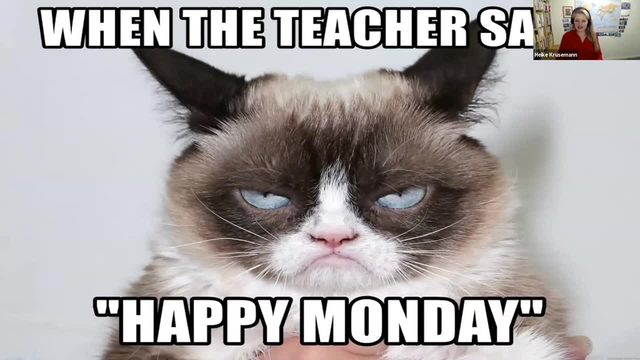 happy Monday everyone. And then all your students are looking at you like this: Okay, so what happened there? Can you type into the chat, which I can now see, just one word that expresses how you think that your students are feeling at that moment with that kind of expression? 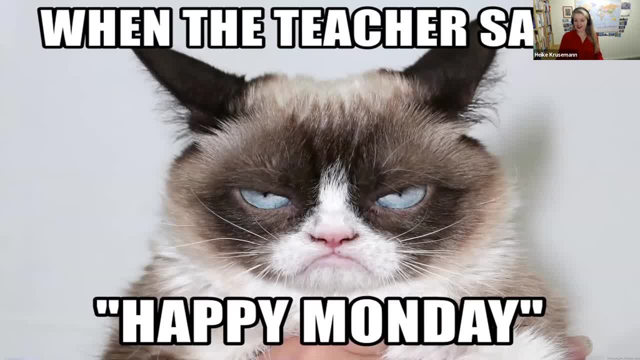 on your face- And I'm getting from your chat that you've all probably been at the receiving end of faces like this. So people say really disgruntled, angry, annoyed, angry, annoyed- quite some quite strong feelings coming up there. So we could tell from your responses that this is 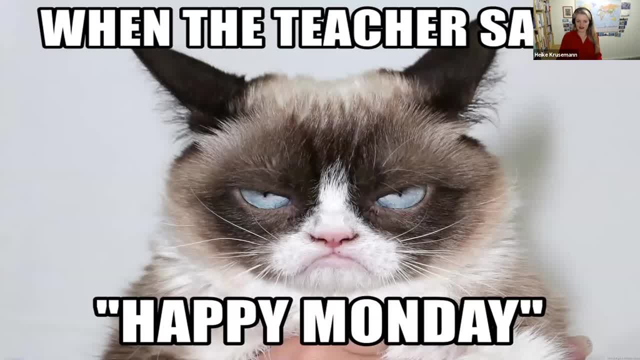 not just a common experience, but there's some real emotions behind that, And so the thing behind this is that it might not be a happy Monday for everyone at all. right, So maybe your students are feeling very unsure of themselves. they have very different things on their mind. maybe they don't. 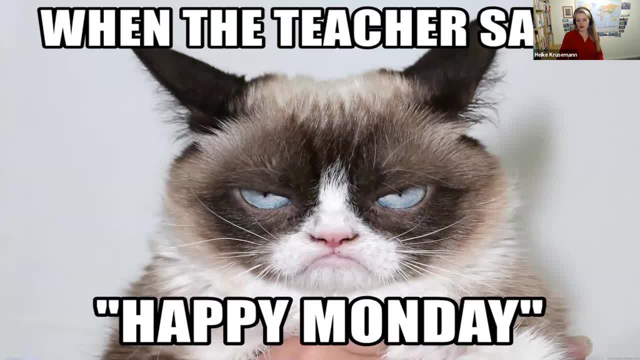 want to even be there at all. they may have even gone through all sorts of difficult situations, maybe some trauma. you don't know, you don't, you don't, you have no idea. so you can't make any assumptions and your mind may be focused on the importance of getting the work done. but your 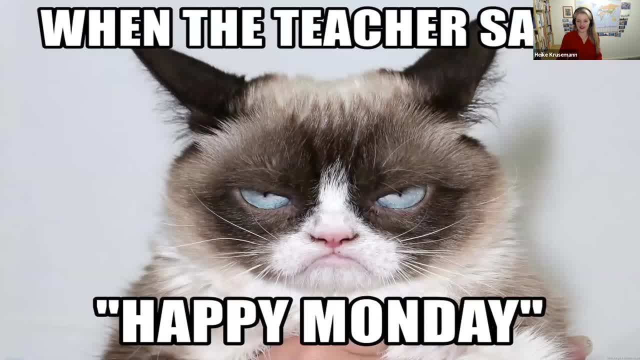 students may not be in the best frame of mind to even take in anything that you're saying to them, let alone engage with any learning tasks that you may give them. so it's very, very important that, when we're thinking about learner engagement, that we start right at the beginning, and that is the 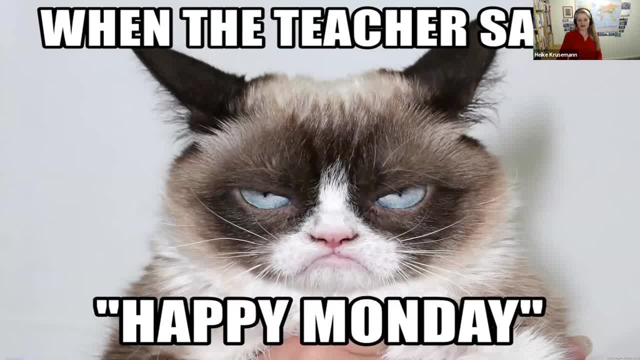 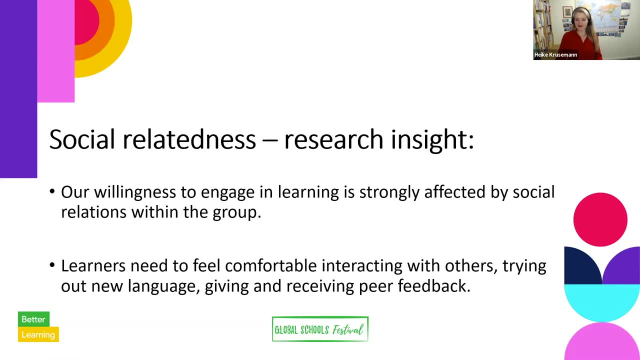 social relatedness among everyone in your class, and that's whether it's online or offline, and I can't stress enough just how important this is. so we know from research that our willingness to engage in learning is strongly affected by the social relations within the group, and that refers 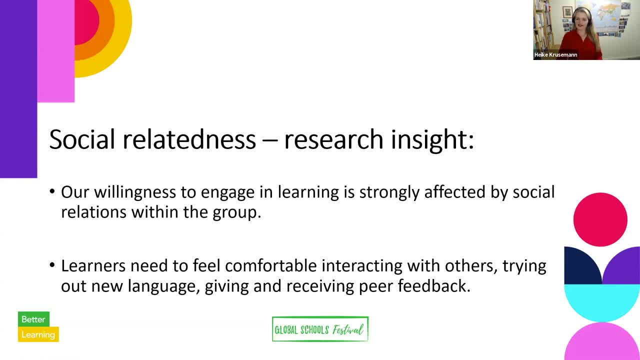 to two relationships. the first one is the relationship between you, as the teacher, and your students. and you can perform the most singing and dancing roadshow with all the latest technology and all the resources if you don't have a good relationship with your students, if your students don't believe. 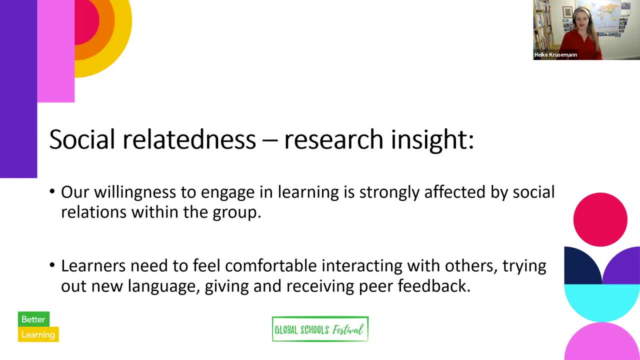 that you genuinely care about them, they are very unlikely to be willing to engage with you and they will probably look back at you very much like grumpy cat that we saw earlier. the second very important aspect of social relatedness is the peer-to-peer relationship amongst the students themselves and learners. they need to. 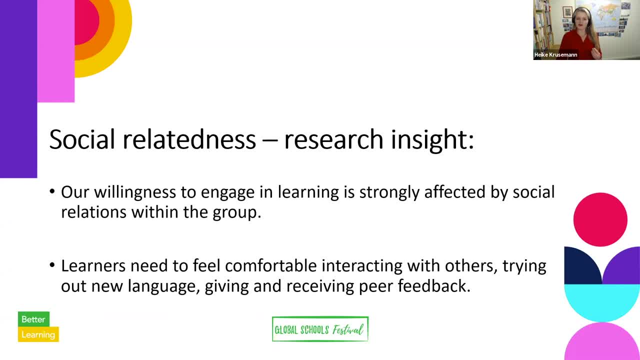 feel comfortable interacting with others in the group so that they feel happy about trying out new language of giving and receiving feedback and studies have shown that students who have a positive relationship with their peers, they also have high levels of engagement, motivation and engagement. so it's very clear from the research and also from our survey findings that 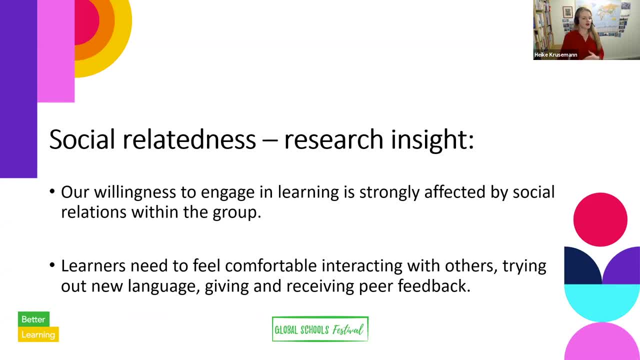 a positive, supportive group culture underpins all learner engagement, and there are a number of features that successful groups have in common, for example, students who may not have a negative or positive relationship with their peers, or those who are engaged with the peers more strongly for some more specific reasons, and we can also feel comfortable interacting with others in the group so that they feel 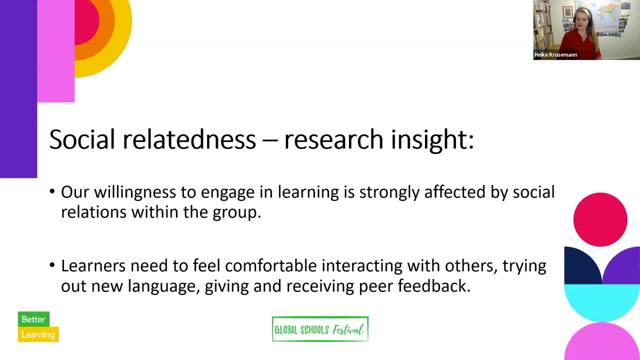 groups have in common and that then you can use to support social relatedness and therefore learner engagement. For example, successful groups have what's called a group legend, and you can support this through maybe a group name or through symbols, a class mascot, maybe a motto or a logo. 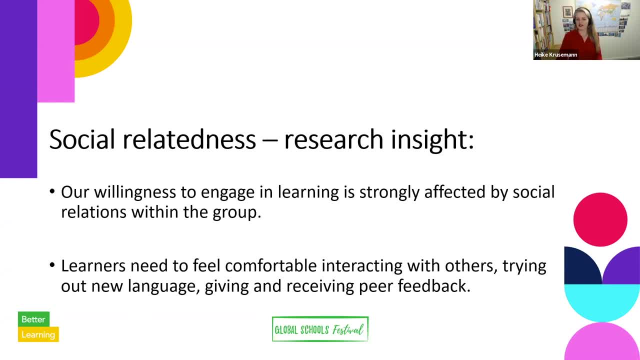 and through this you're creating a sense of belonging and trust amongst the group members. and if you can think of other ways of supporting group culture in your particular teaching context, then do feel free to share that in the chat. Okay, something else you can do to support? 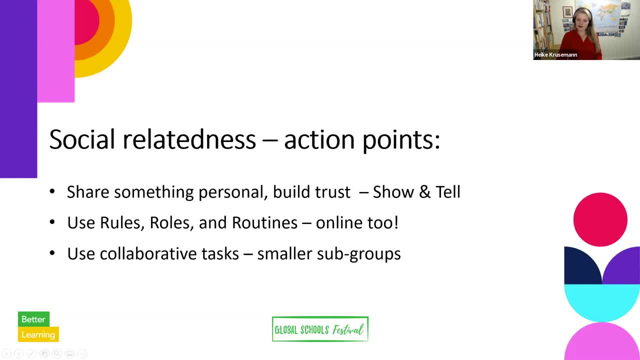 the social-emotional climate in the group, then, is to share something personal with your students, and this builds a relationship of trust. So I would say, encourage your learners to share something appropriate with the rest of the class, So, for example, you could invite them to bring in an 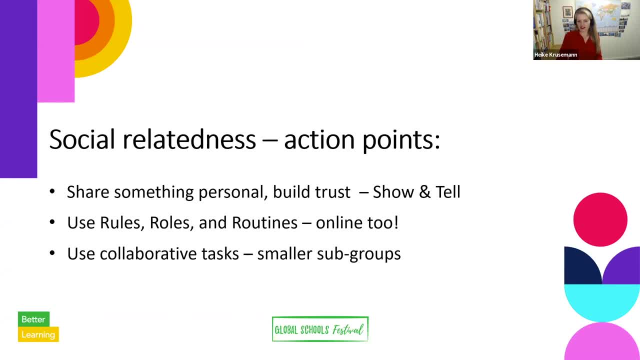 object and talk about it for a minute. that's often called a show-and-tell kind of activities and these are great for success. SHARE-ING OF THE CLASS- these kind of activities are really great because they also work very well online in a whole group. 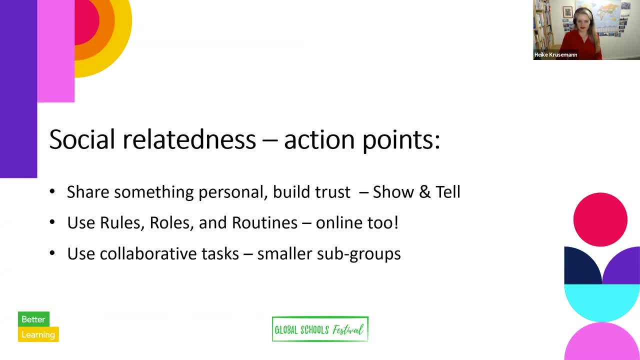 or you could use breakout rooms and of course, they was to work face to face. so, for example, I like to travel, which you've probably guessed based on the big map of the world behind me, surrounded by postcards. not that there's much traveling going on at the moment, but I might. 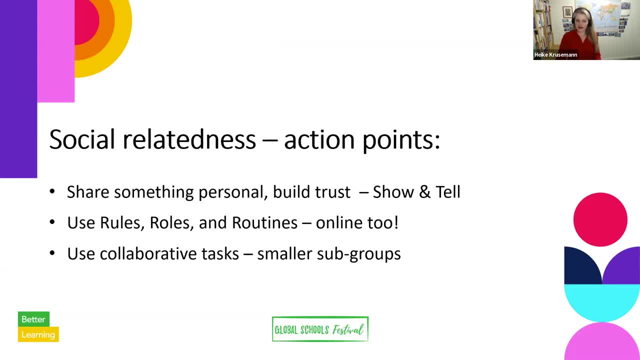 still show my class a postcard and I might start a discussion that way, and then postcards are a really good hook for creating a talking point and you can even start a class collection of postcards or any picture cards that learners can bring in that they have an interest in, that they. 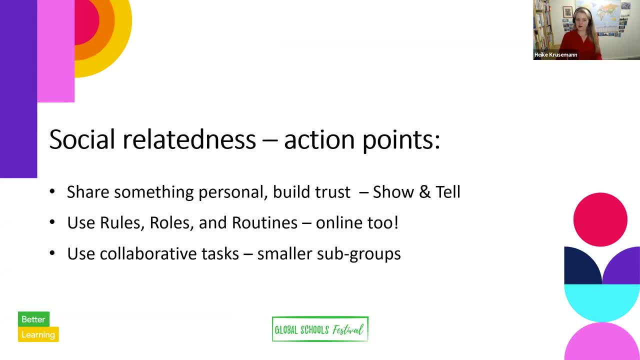 want to talk about, and this would be a great way to share something personal, which strengthens connections within the class. Second, it's also very much worth thinking about what is referred to as the three R's, and the three R's I mean here they stand. here, the R stands for rules. 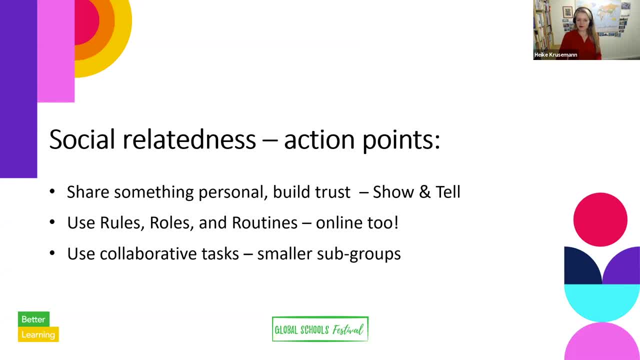 roles and routines, And it's especially important to think about rules afresh for managing the face-to-face classroom in a socially distanced way, as many of us are having to do, and so you can use this new context that we find ourselves in to involve your students in discussing those rules and why. 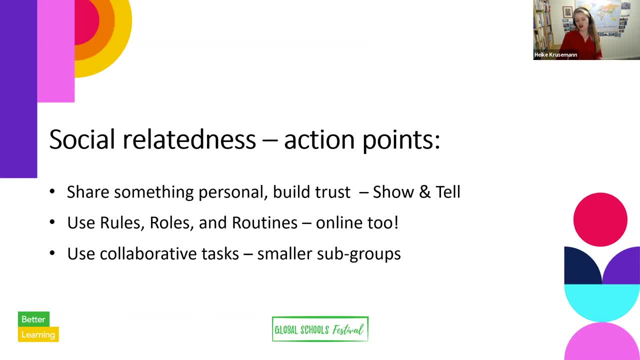 they are necessary and that they are there to keep everybody safe- again showing your students that you care about them. Roles are helpful for students to concentrate on a specific responsibility so you can work with your students and you can work with your students and you can work with your students. 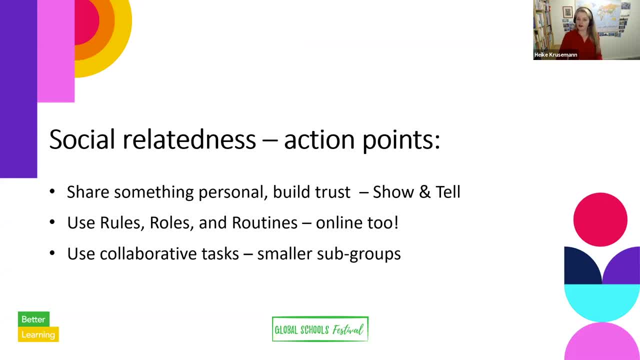 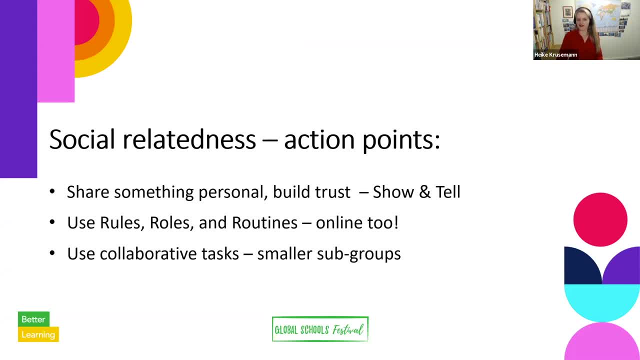 skills, For example, so that you could assign the roles of affect checker or a summarizer, or a notetaker, a spokesperson, a timekeeper and so on. all these different roles, And the last R stands forX routines. so routines really help to provide structure and security and 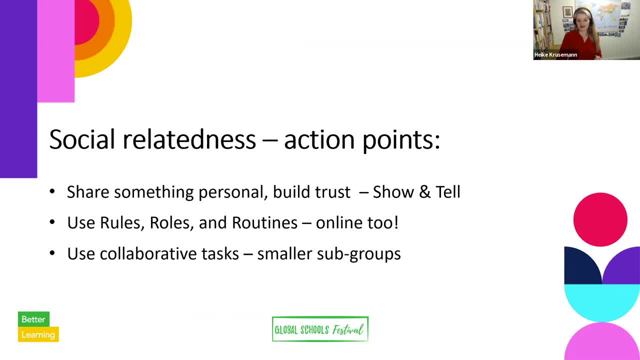 this is especially important when things feel uncertain, as they may do now, and it helps to helps everyone feel a little less overwhelmed. And all of these three R's of rules, rows and routines- they can be implemented very well online as well as in the face to face. 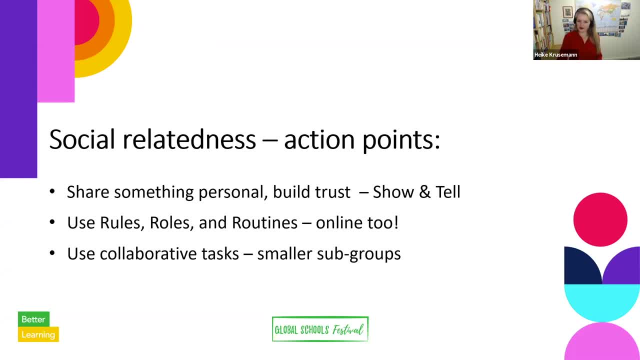 classroom. And the third action point for supporting social relatedness is to use collaborative tasks as much as possible And using smaller groups or even just pairs online and breakout rooms or face to face. this is a good way to strengthen bonds between learners And it also teaches. 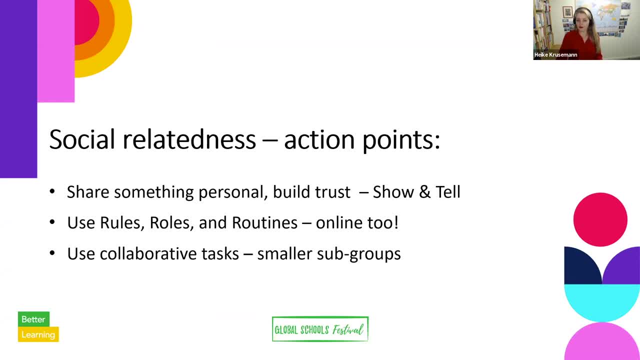 students collaboration skills, And this is a key life competency, And this will come in useful much beyond your language class as well. Now, one idea for the socially distanced classroom, where you can't have learners moving around, you can't have them being in close proximity to each other, would. 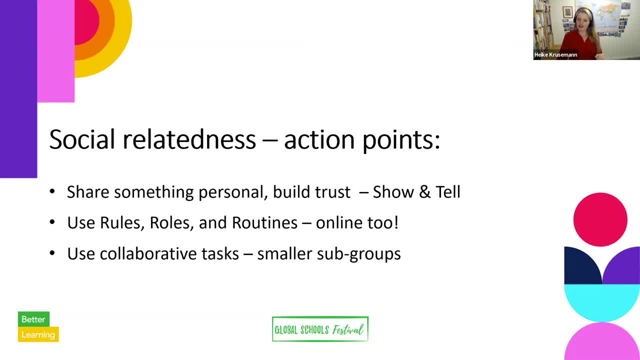 be to have the whole group stay where they are, But you could single out individual learners dotted around the classroom and maybe give them a colored card each so that they know which group that they're in. And then who else, maybe three rows behind? 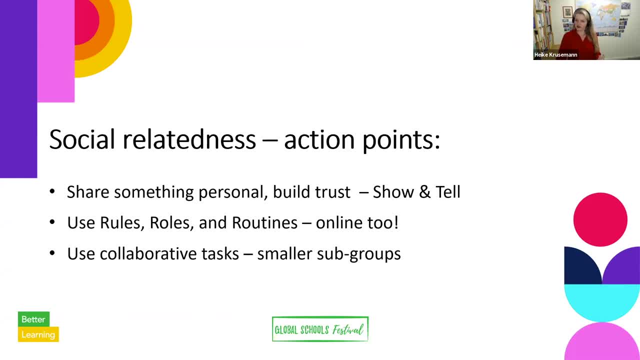 And then the person behind them is also in that group and so on, because they'd be identified by the color of their card And then they can do the task out loud while the rest of the class listen and make notes. And then another group with different. 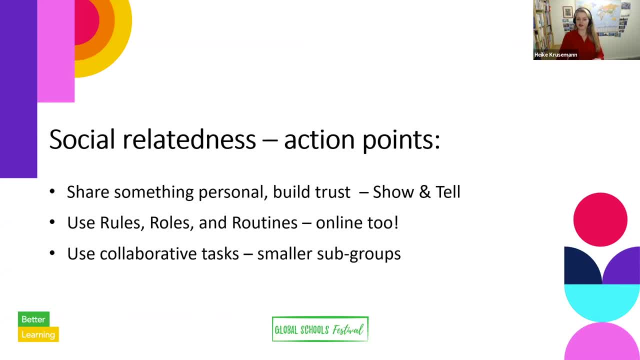 color cards can do the same until every student has been involved, And then you can open up a whole group discussion after that. So I would like to invite you now to suggest, by typing into the chat, what kind of activities you think would work in your own context. 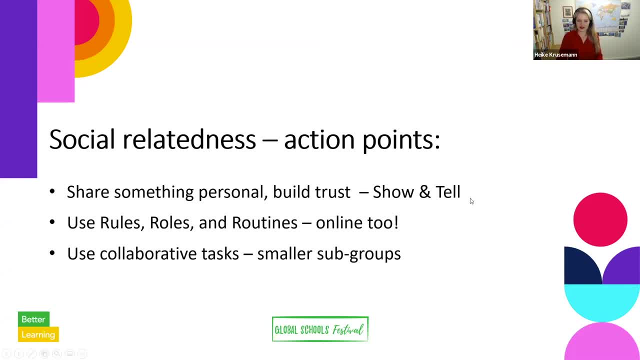 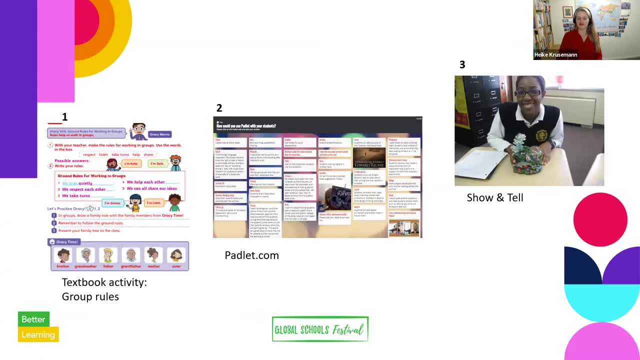 to strengthen teacher-student rapport and to build positive group dynamics. And while you're thinking and typing, I've put just a few examples here of activities that may do that. So number one represents setting up group rules, And two is using the Padlet tool for whole class collaboration, And you could also 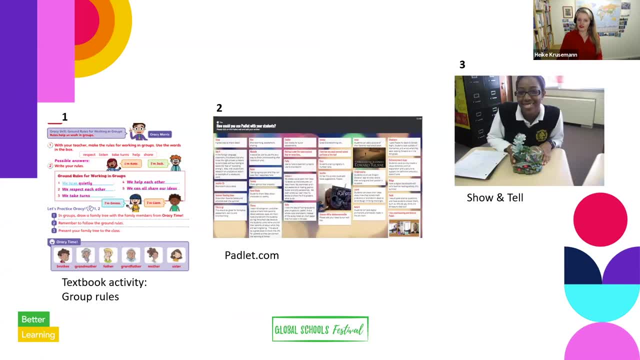 use this to build a class wall, And this would be helpful for representing visually a group identity. And three is sharing something personal In a show and tell type of activity, And this would- these would just be a few examples of activities- that strengthens that. 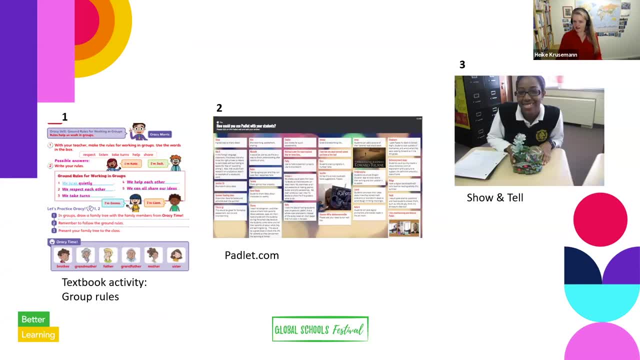 strengthen the social relatedness in your class. So people are typing yes. Quizlet personal profile can see that discussion creator doing trips together. Yes, maybe, maybe in a little while. maybe he could ask students to imagine doing a trip. 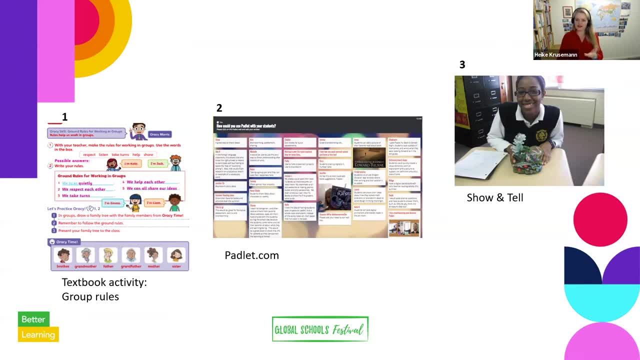 to together and write about it, do a little video about it. These are all really great, Great, great suggestions that you can use in times when you can't actually do any physical travel. Okay, another key building block of learner engagement, then, is self. 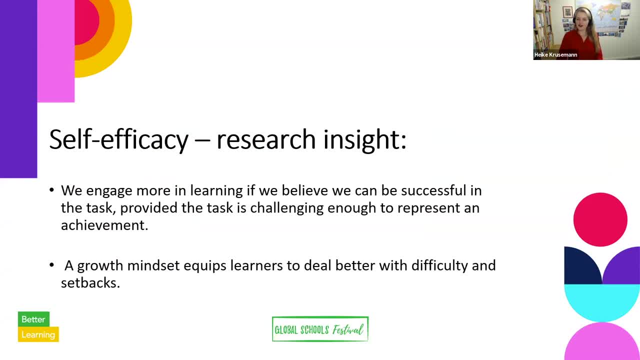 efficacy. Now, self efficacy means a belief of I can do it, And research tells us that we engage more in learning if we believe that we can be successful in the task. And for this it is very important that the task is just challenging enough to be manageable, but still. 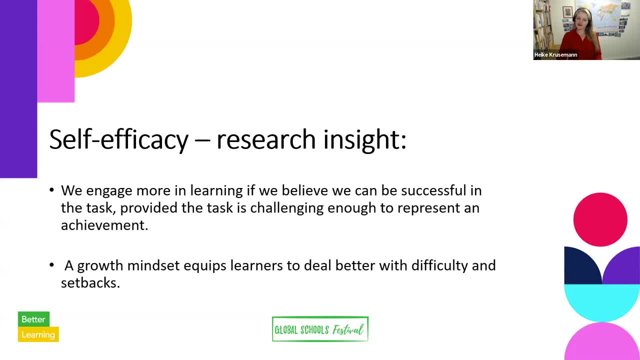 represent an achievement. And also tied in with this notion of self efficacy is the idea of a growth mindset, And a growth mindset means a belief that improvement is possible, And it's this belief which enables learners to deal better with difficulty and with setbacks if they frame them as a challenge. 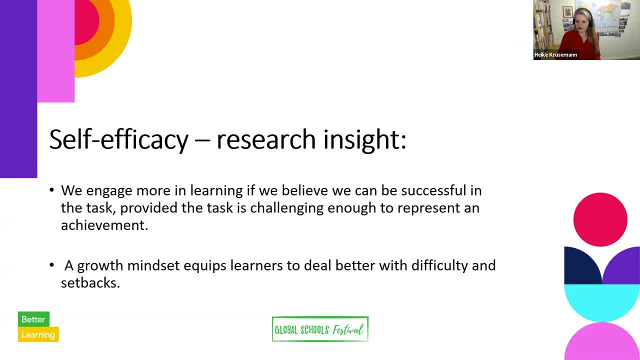 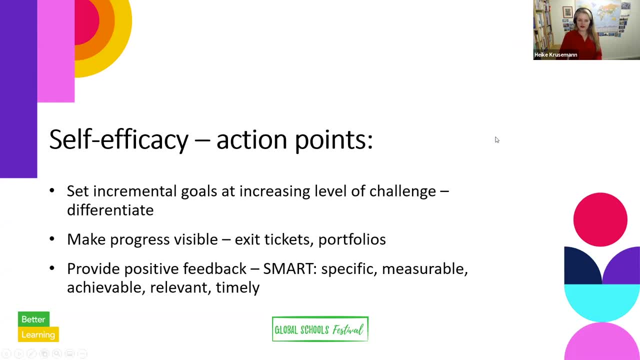 that can be overcome. So what do we need to do to support learner self efficacy? Right, we need to provide plentiful opportunities for success, And you can do that by setting incremental goals at increasing level of challenge, so that you give your learners the confidence that they can be. 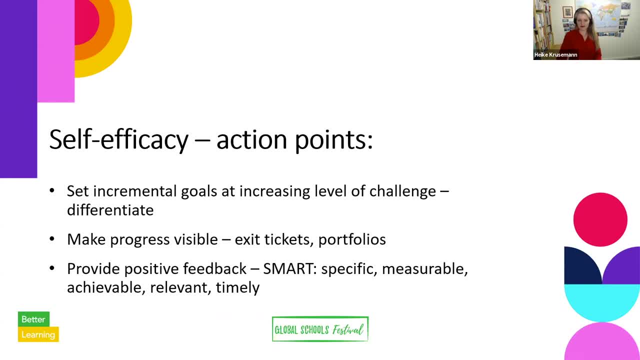 successful at a task by staggering achievements, And for this you will most likely use differentiation, And I'm aware here that often teachers hearts sink at the mention of the word differentiation, because teachers tend to think this means extra work and they really don't have the time for any more extra work. 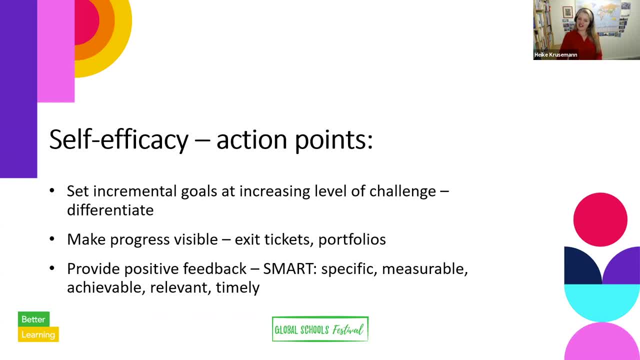 And I understand that. But don't worry, because differentiation doesn't have to mean extra work for you. So, for example, you could set a reading task where the text and the questions are getting increasingly more challenging, And then you could say to learners: 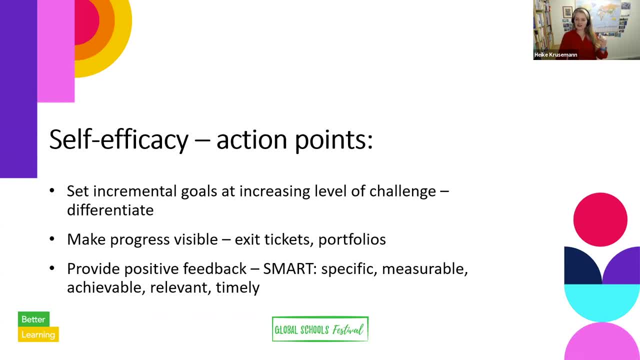 okay, so we've got one text here, but the text starts off easy and then it gets harder with each paragraph, So I would like you to choose where you start. So look at paragraph one, And if that's too easy for you, then you go to paragraph two. 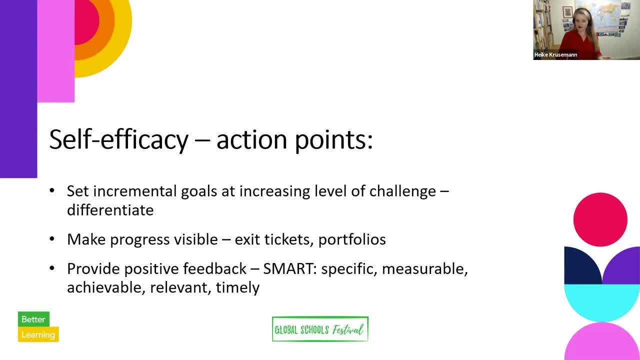 and you start there, And if you're feeling even more confident, then start with paragraph three, three or four and so on. So you choose your own starting point And in that way you, as a teacher, you've only had to design one single. 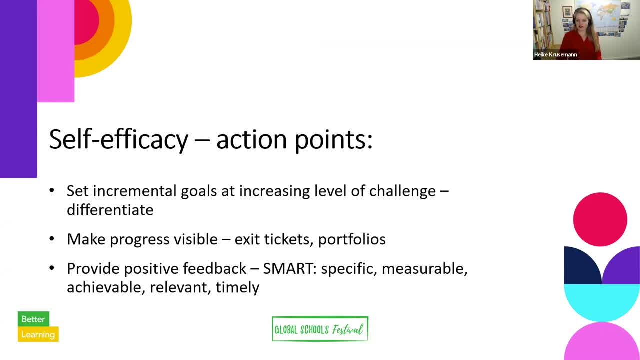 activity for the whole class, So no extra work. it saves you lots of preparation time, And so this activity builds the challenge up in incremental steps. It also offers a differentiation: with no extra work And because you're offering learners a choice, you're also supporting another key factor for engagement, which we will come to. 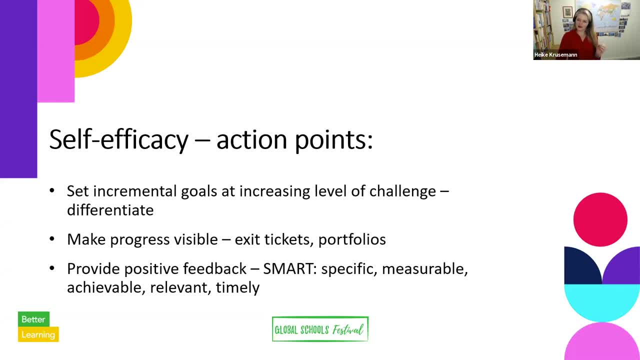 Very shortly Right. the second action point for self-efficacy is to make progress visible Now. sometimes it's hard for learners to see how far they've come already, And you can help build their confidence by visualizing their achievements, And it's. 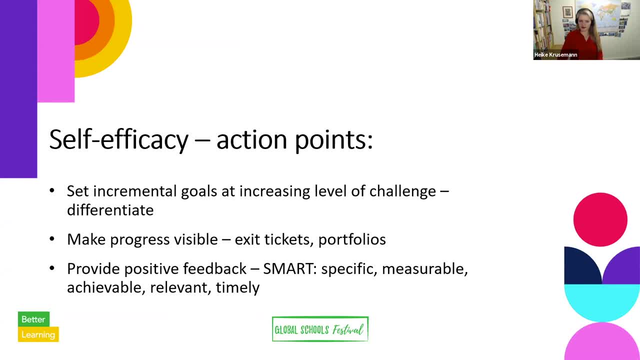 really important to celebrate small wins as well, not just the big milestones, And a few ways in which you could do this, for example, through a traffic light system of having a blue, amber and red, or through exit guidance, So you could do this, for example. 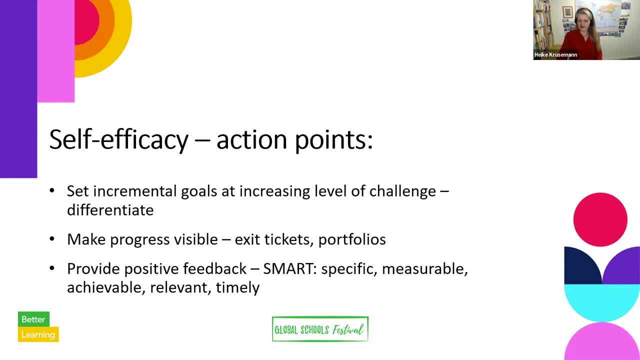 through a traffic light system of having a blue, amber and red or through exit guidance. So you could do this, for example, through a traffic light system of having a blue, amber and red, or through a traffic ticket tickets where learners rate their understanding. 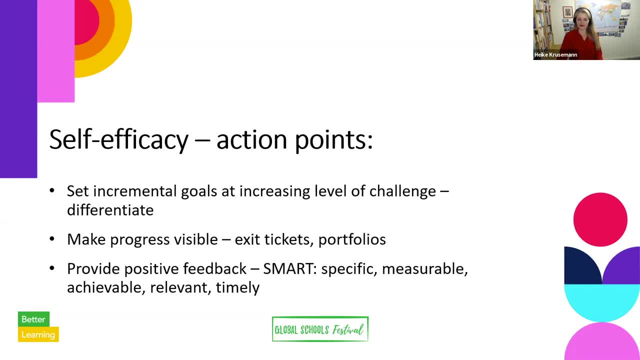 of the lesson. For example, you get some free software like the assessment tool. Socrative formative assessment tool does this very well. Or you could use student portfolios, where students collect samples of their work throughout the course And it's extremely satisfying to flick back to through all your work and 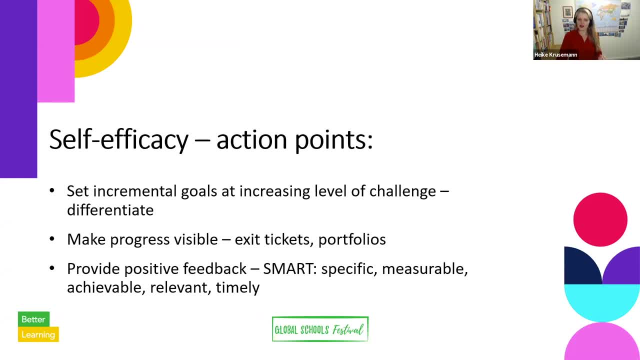 to look back on what you've achieved already. it's a really good visual reminder, And this can be done on paper and displayed on the class, but it can also be done online using digital tools. Last is feedback. Now, feedback is crucial. 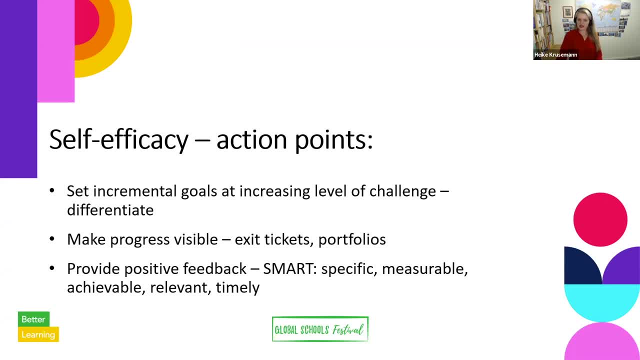 to get right. And to my mind, the most important thing about feedback is that it should be encouraging for learners and it should be meaningful. And that means it's not good enough to say to learners, well done, good job, and then move on. just to be encouraging. 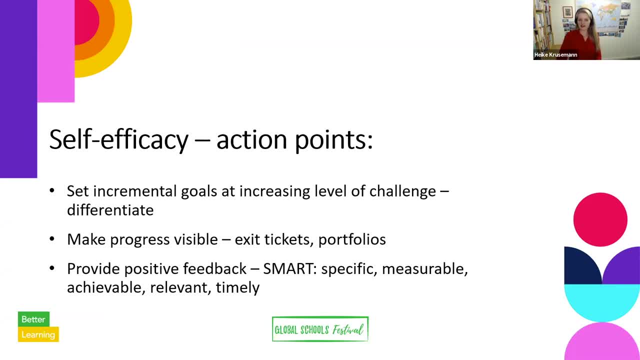 But it's a good idea to use SMART criteria- S-M-A-R-T, Now SMART. we've all heard this and probably not always love this when it comes to our own goal setting for CPD, But I think it works extremely well for feedback. So here's a reminder that we've got to be. 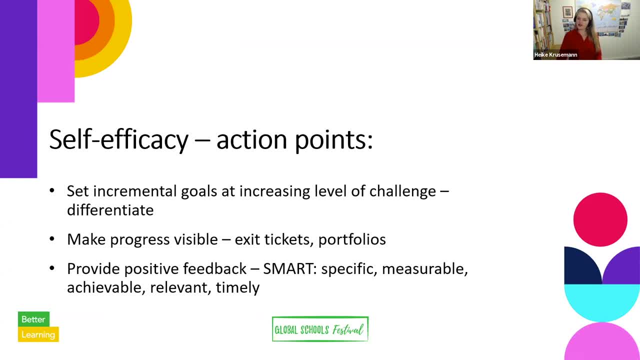 specific. in our feedback to learners, We have to set measurable and achievable goals. The feedback has to be relevant And it's got to be delivered in a timely manner so that the window of opportunity for learning is not lost. Right Now, all this task of instilling. 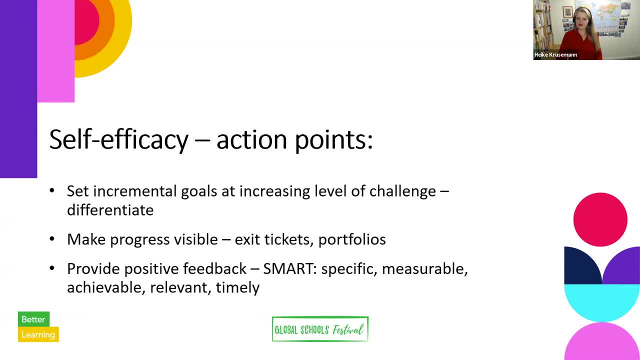 a growth mindset, an I can do it mindset in learners. that might remind you a little bit of positive psychology, focusing on encouraging self-talk and attitudes, and you would not be wrong in thinking that. But there's also a slight danger in this way of 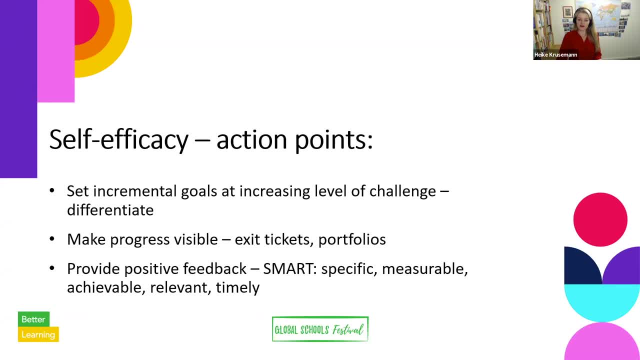 thinking in that if you're not careful, then envisaging positive outcomes it can feel a little bit like wishful thinking, And there's actually some research which shows that if people dream too much about achieving their goals, they actually achieve less than if they didn't do. 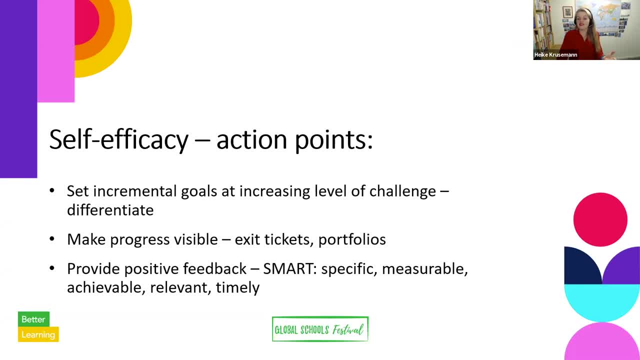 this, And that's because if in their dreams they're already there, they've already achieved their goal, then they may feel less of a drive in real life to move them, to put in the effort required to actually make things happen. So 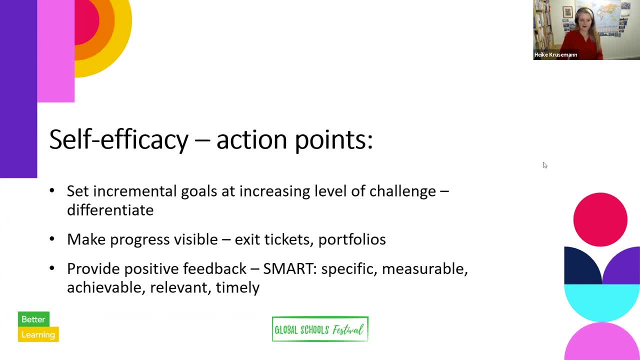 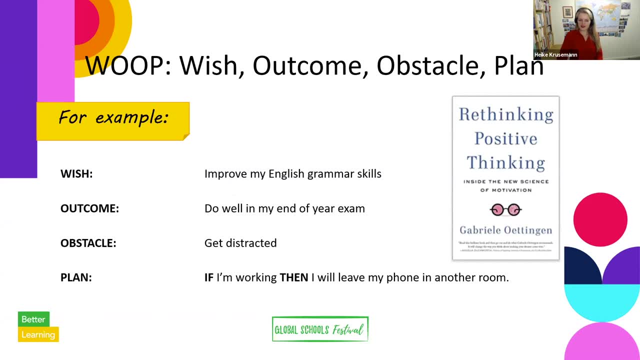 I would like to share with you a goal setting tool that I really like, and that is the WHOOP tool developed by Professor Gabrielle Oettingen, And that's from her book Rethinking, Positive Thinking, And again, you will find the full reference at the end of my slides. Now, WHOOP. 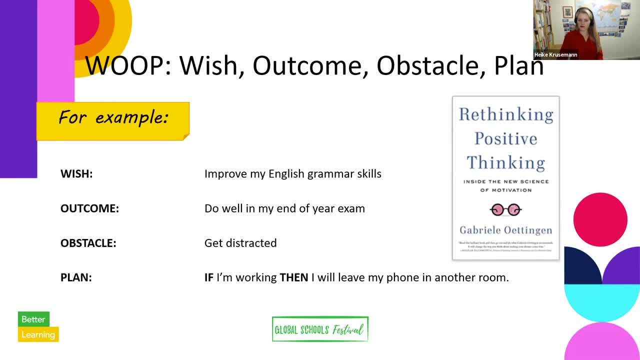 is an acronym and that stands for Wish Outcome Opset, And you can use this with your students for achieving their goals by helping them to anticipate obstacles to their learning and then identify strategies to overcome these. So, for example, a student's wish could be to improve their grammar skills, And then the outcome would be they'd 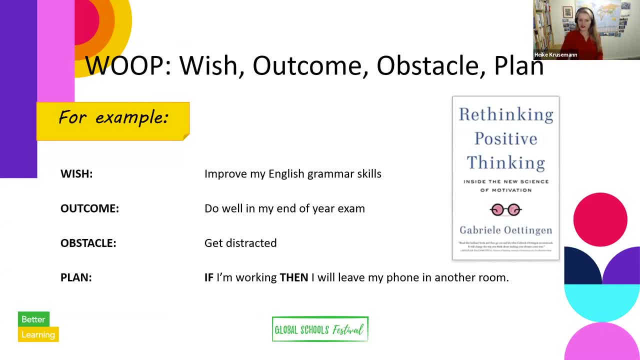 do well in their end of year exam. And now, when it comes to the obstacle, it's a very important rule that you're only allowed to list something inside of you that is stopping you from achieving your goal, And this is something that we've been talking about in our learning sessions today. So if you're 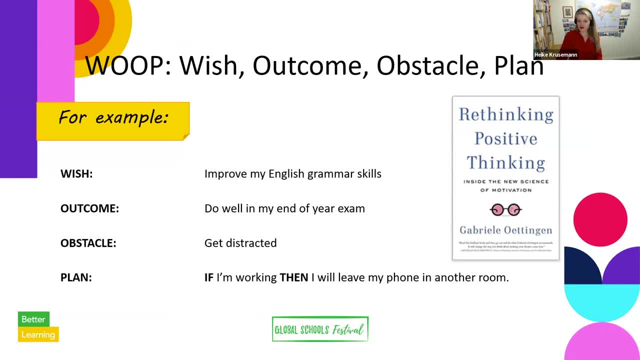 way of thinking, does away with all the excuses that we're all in the habit of making of why something can't be done. And the idea is that once you've realized it was you who put the obstacle there in the first place, then you can also overcome it, And you can overcome it by setting 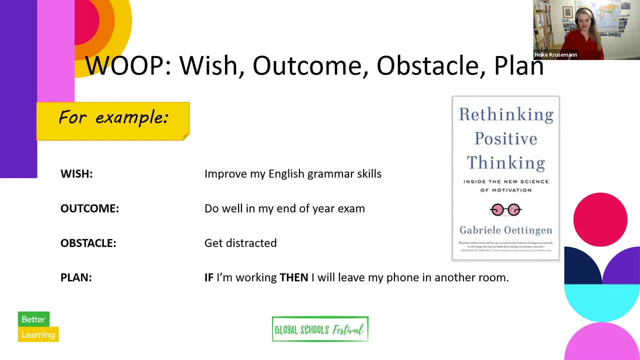 a path to action with an if-then scenario. So an example for myself would be: I also get easily distracted by alerts coming up on my phone, And two of my favorite phone apps that can really set my attention are Twitter and Instagram. So I've made a rule for myself that if I'm working, then 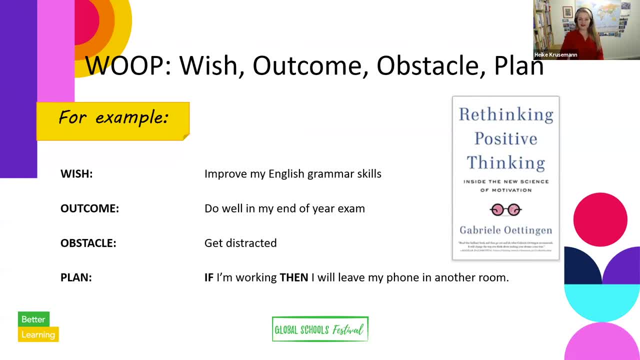 I will leave my phone in another room And maybe you can also think of some ways in which you can use the Whoop tool with your students to help them not just to set but also to achieve their goals And, like me, then you may find that it also works for yourself and your own goals. 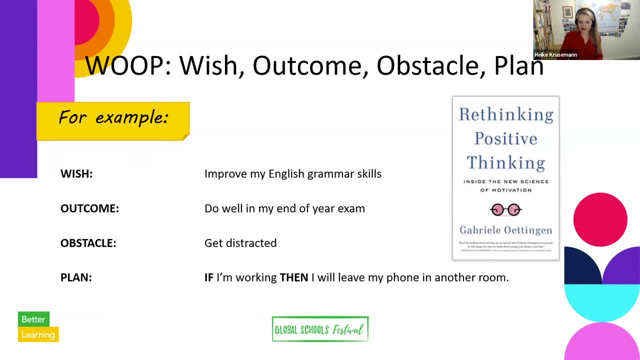 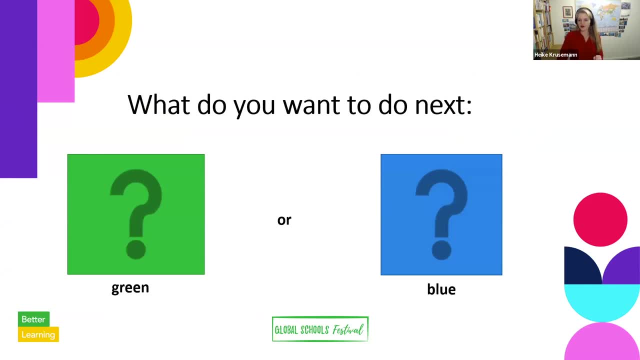 Right next up. I have a question for you And I'm giving you a choice now of what you would like to do next, And the choice is: what do you want to do next? The choice is green or blue, And we've got a little poll prepared for. 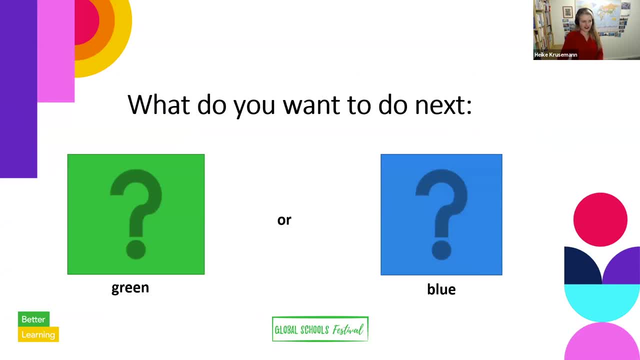 you now And, Eve, if I can ask you to start the poll Now, I have to apologize. If you're watching on Facebook Live then I don't think you can see the poll, So instead just type in the word green. 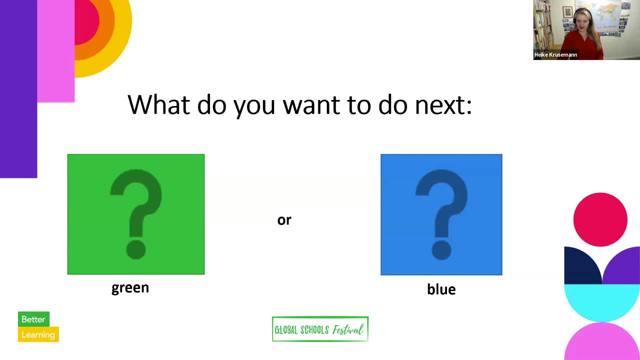 or blue into the chat. You can do that as well, And I'll keep an eye for that. So the choice of what we want to do next is green or blue, And I'm just going to count down from five And then Eve's. 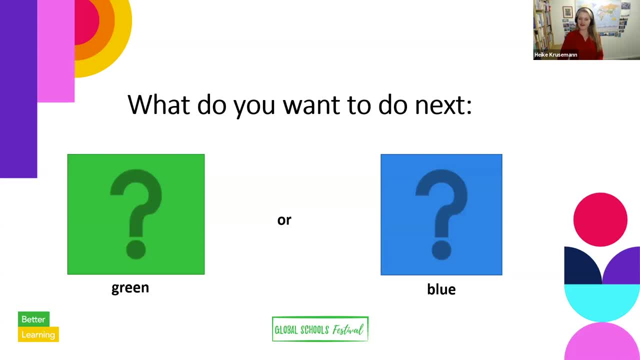 going to close the poll And I'm going to share the results. So I'm going to close the poll And I'm going to share the results with you. So we go five, four, three, two, one And Eve, if you could. 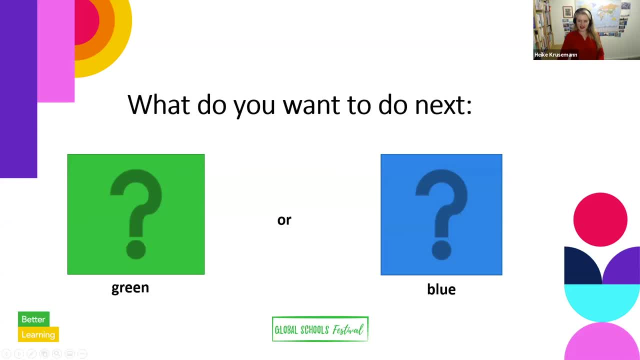 close the poll, And I can tell you, looking at the chat and also at the poll, that 61% of you voted for green. Okay, so thank you very much. That was the end of our little poll, So the majority voted. 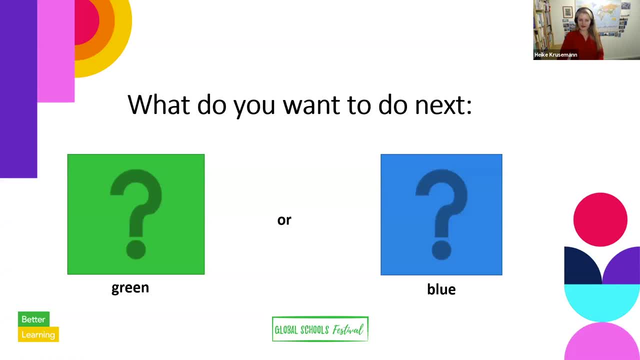 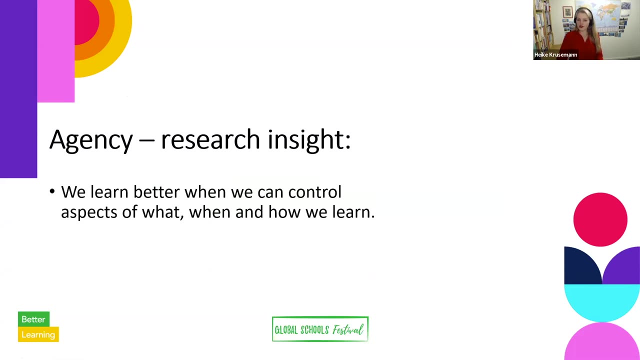 for green. And so this brings us to the next building block. The next building block of learner engagement, then, which is agency, And research into agency tells us that we learn better when we can control aspects of what, when and how we learn, And this 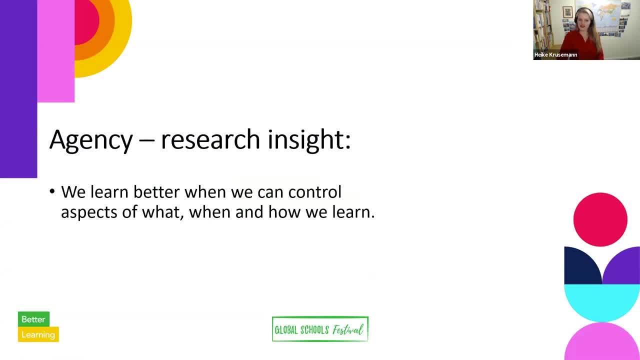 is what I was referring to just a moment ago when I talked about the activity using differentiation, where learners could choose their own starting level. And maybe take a moment to notice how you were feeling just then when I offered you a choice. So you were exercising. 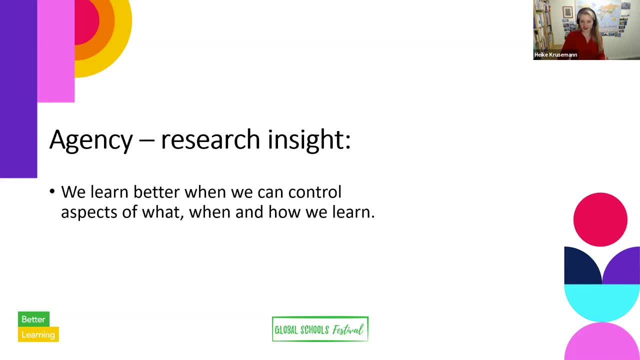 your agency and you didn't even know really what it was about, what the choice was about, but you still participated. And so have a think how that made you feel and how you can use that to empower your learners in that way, So in your teaching, wherever possible. 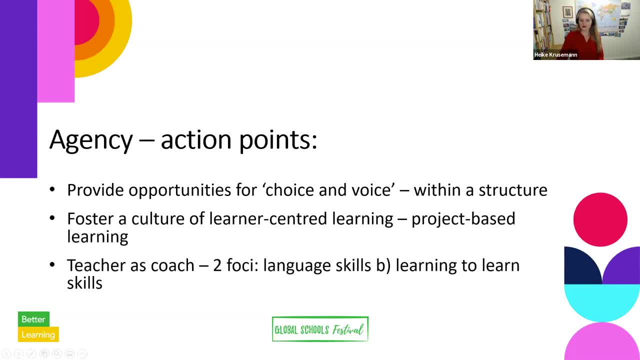 provide opportunities for choice and voice, And I really like this phrase because it expresses in a very clear way what we should try and build into our teaching. But two things. One is that too much choice can feel overwhelming, So to avoid making choices too overwhelming. 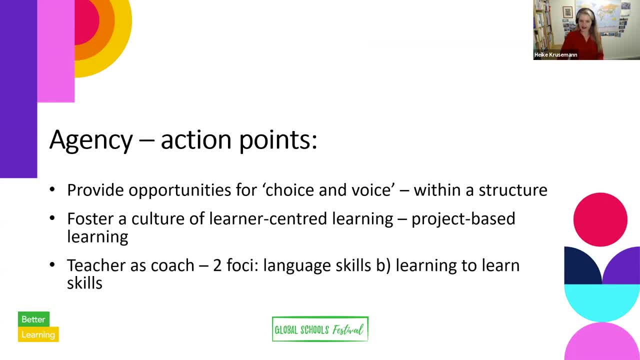 it's a good idea to keep them contained within a structure, And an example of that might be that for a writing task, you could offer students two options, So, for example, they could write a formal letter or be an informal text message, but they would both both these forms of writing. 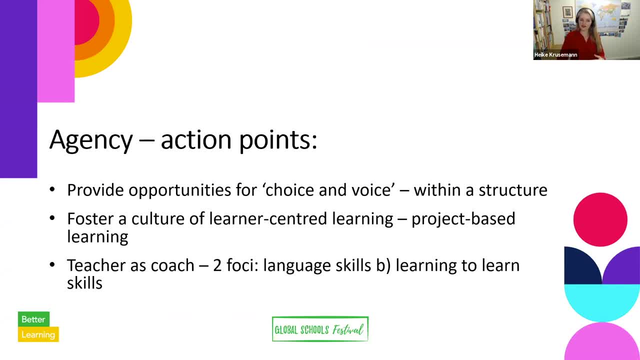 would express the same content, Or you could keep the format the same and offer a choice, a choice on the content content. So, for example, the task task could be to write a blog post to persuade readers to donate to charity, but you could let choose students choose a charity that. 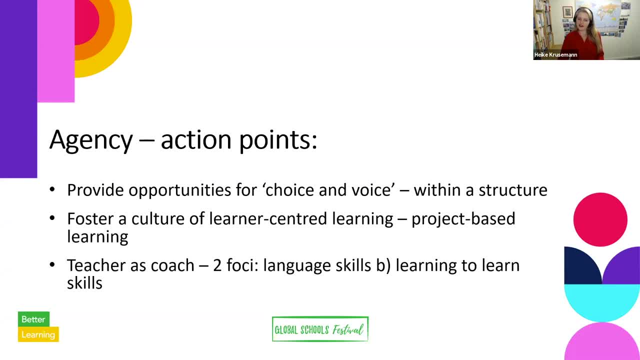 they would want people to support. And the second point: to support support learner agency says that we want to do. we want to foster a culture of learner centered learning And for this, project based learning is ideal And that's because projects put puts, projects put learners. 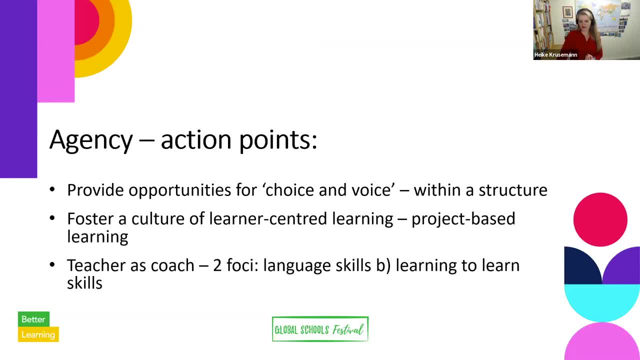 in an active role and allow them to make decisions. and if you're involved in a project and you have a very specific role and very tangible outcomes, like acting in a play, for example- you can't just sit there and let things wash over you. you just have to participate, you have to engage through. 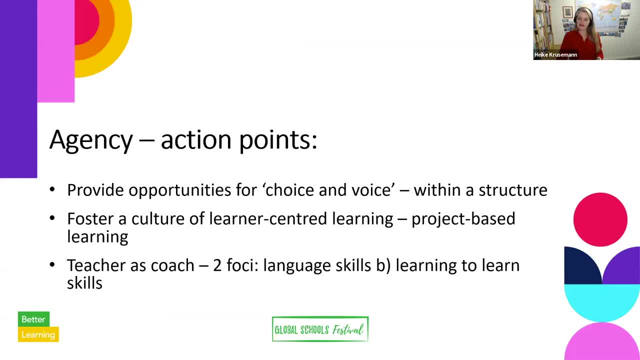 the very nature of the task. and last, think of yourself as a coach rather than as a teacher. now, this is a bit of a mental shift and how often, how we often traditionally think of ourselves as teachers. but it might be helpful to think about that if we want to think of the learner as at the 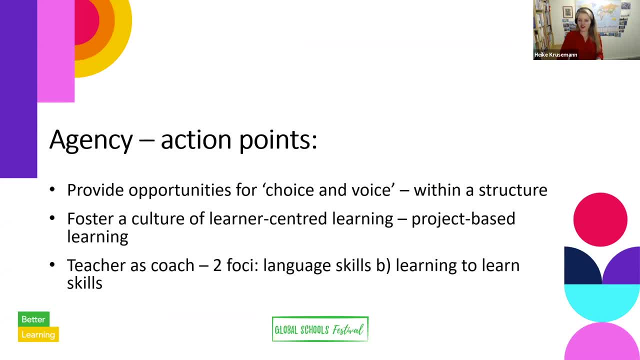 center of their learning, then this means that we as the teacher, we can't be in the center. we have to move a little bit away from center stage to make room for the learner right, and so for us it's to support the learner from the sidelines more like a coach and in the classroom. this means not 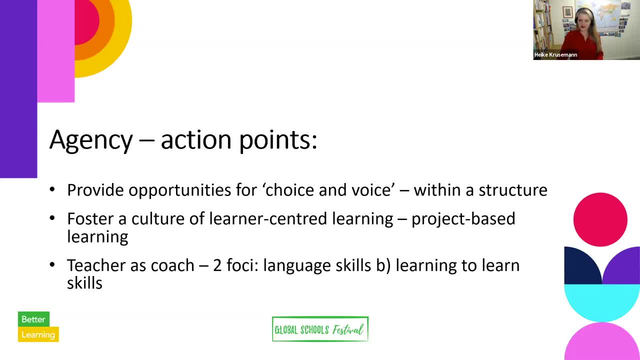 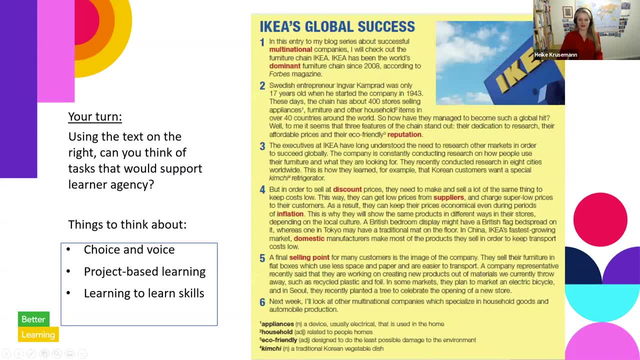 a reading text, and that's the text here on the in the yellow background. now there is no need to actually read the whole text. if you can't quite make that out on the screen that you're watching, then don't worry about that. it is really just to give you an idea of the kind of source text that 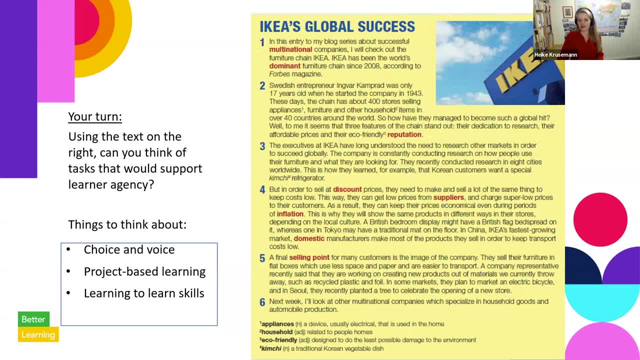 might typically be used in teaching, and that's what we're going to do today. so let's get started. first of all, let's get started. so we're going to be talking about a text that kind of forms part of a structure, of a machine learning. so this text is which does not attract the needs of 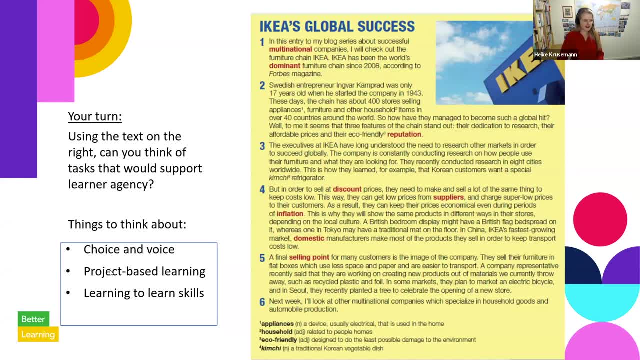 the students, as it does indeed also draws on the understanding of language and the needs of the students to help them develop their thinking skills, and that's what it is about, and that's exactly what we're going to be doing today, and it's going to be about the understanding of language. 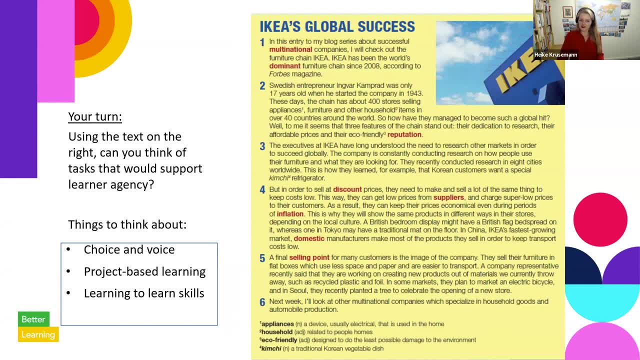 and the needs of the students and we're going to try to come up with a little more detailed material, and that's what we're going to do today. i'm going to go through the course a little bit: how you could use this reading text, or a text like it, to increase learner engagement through. 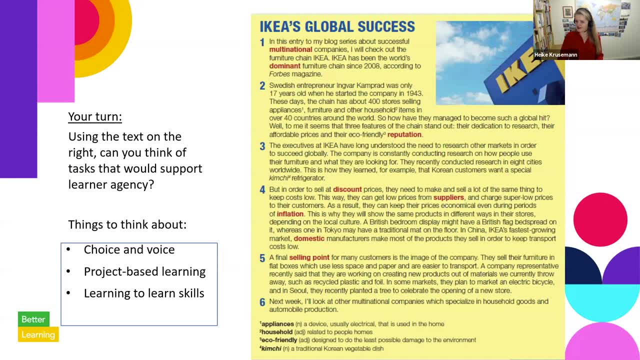 supporting aspects of learner agency. Okay, so I can see people typing jigsaw reading. That's a really good idea. Yeah, who reads what? Scanning a text for new words: Yes, more of a language focus Role play from the text. changing the format: Yeah, that's a very good idea. So some excellent 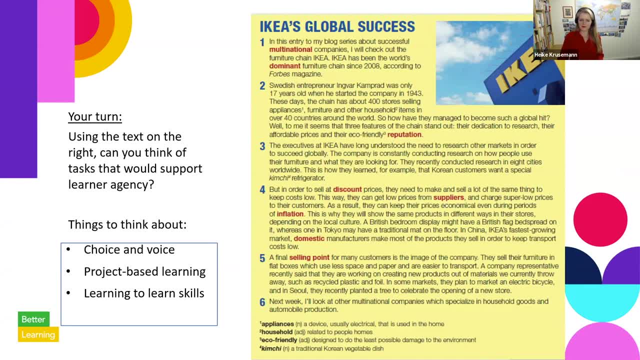 ideas coming up there from everybody And so for choice and voice. you can see that the paragraphs here are numbered- And I really love numbering paragraphs- And, like in the example that I used for self-efficacy earlier, to give learners a choice which paragraph that they like. 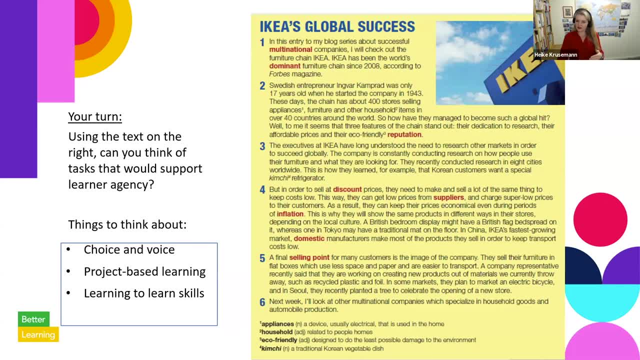 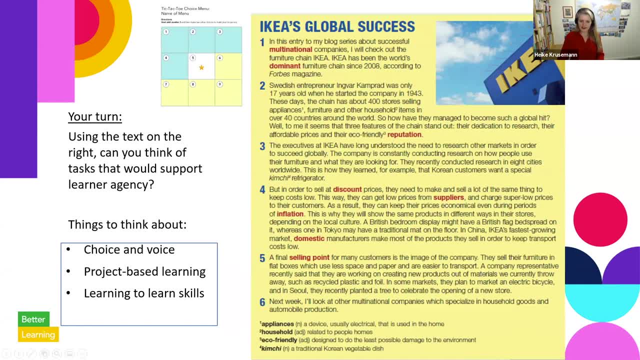 So for offering a choice, you could design a choice board like this one here, And it's like a noughts and crosses, or sometimes also called a tic tac toe style board, And you can put a task in each box And then learners can choose a task from each row. So again, it offers a choice, but within. 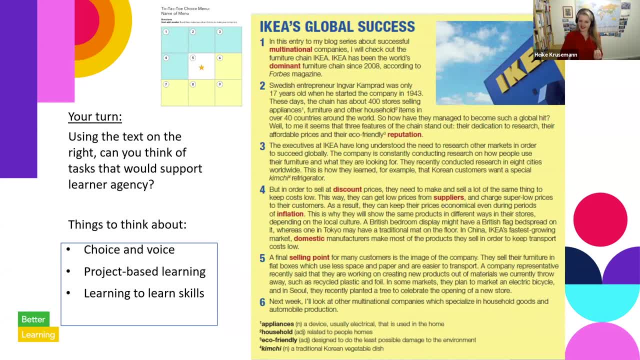 a structure And for the middle box. you see, there's a star in the middle box And you could ask learners to come up with an idea for a task themselves, And this would be an opportunity for your learners to express their voice, And then you could also put a task in each box, And then you 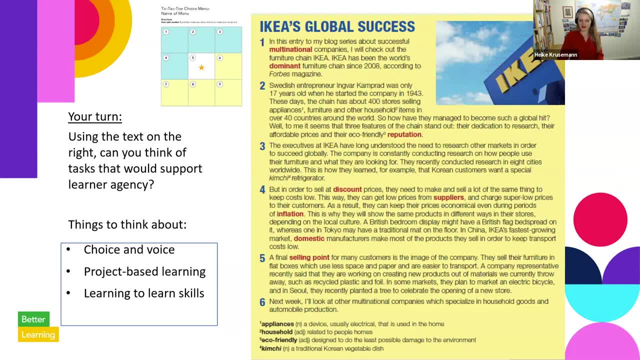 could also put a task in each box, And then you could also put a task in each box And also make a meaningful contribution to the learning process. And another idea for voice is that you could offer your learners the opportunity to express their opinions as part of the learning tasks. 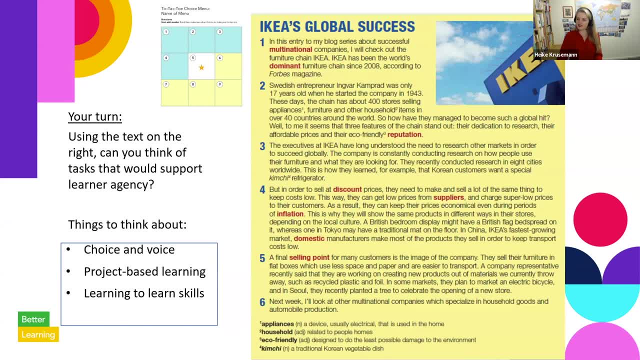 exploiting your source text. Now people are typing about project based learning. that's really good idea. So you could use this text and build it into a larger project where groups of learners can choose their own focus. So it could be, for example, around multi. 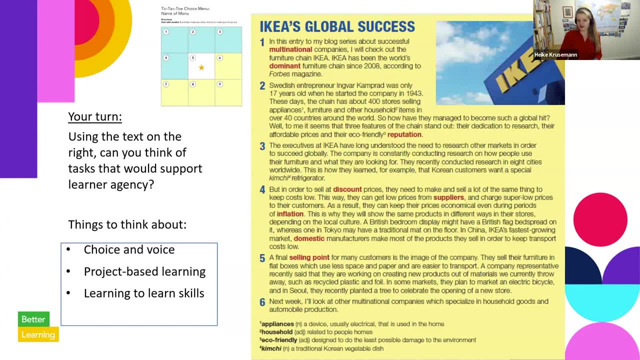 national companies, around marketing, around environmental concerns. it could also be a language focus, such as giving instructions using the example of putting up flat pack furniture, that kind of thing. All of this is rooted in a real life situation And that's usually at the 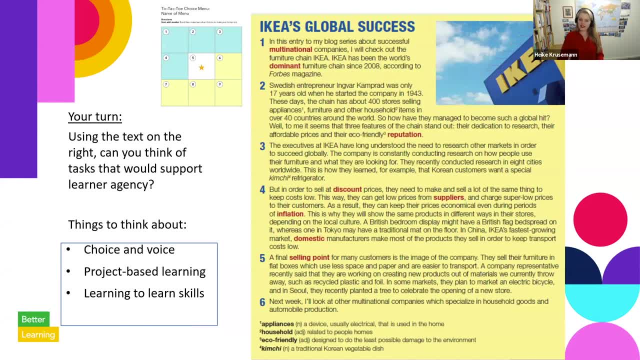 heart of project based learning And for learning to learn. one way in which you could address this is to teach students decoding strategies. So to pay attention to clues from the title- people already pointed that out- from the images. to work out meaning based on the adjoining words, using 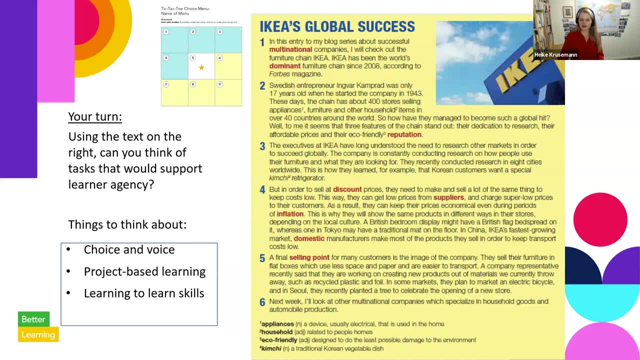 the context using the code text of words, and also to use their knowledge of their first language or from other languages. And all of this is providing them with a repertoire of strategies that they can use to exercise the agency so that they can make choices which will engage them more. 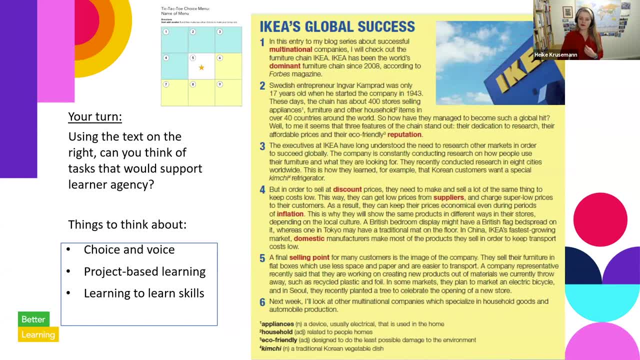 fully Okay. so we were talking about real life situations being at the heart of project based learning, And this brings us to the next building block of engagement, which is relevance, And the research insight here is that we are so much more motivated to engage. 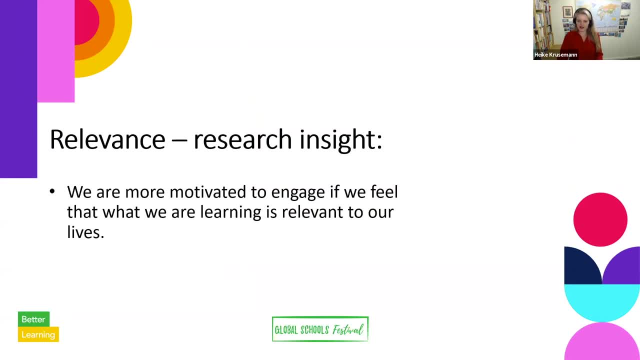 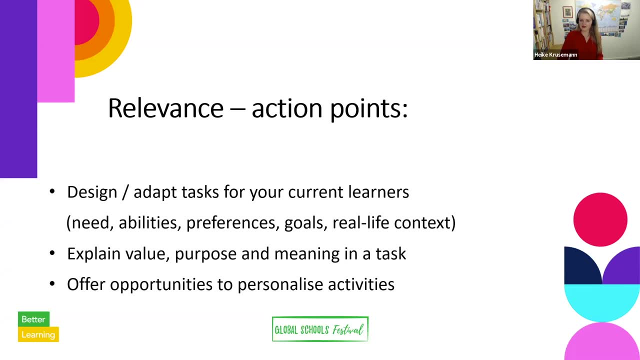 when we feel that what we're learning is relevant to our personal lives, And this means that it's very important that we design, or at the very least adapt, tasks for the learners that we're currently teaching. And, don't worry, this does not mean reinventing the wheel every time we start teaching. 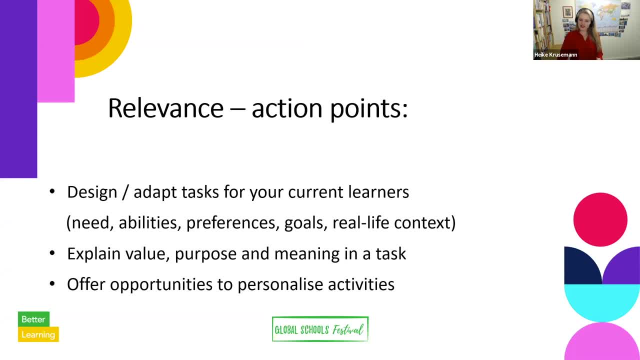 a new group. Sometimes it can just mean making a very small but effective tweak to our existing materials, And one technique that has worked very well for me in the past is that when you're planning a lesson, then focus on just one or two particular students in your 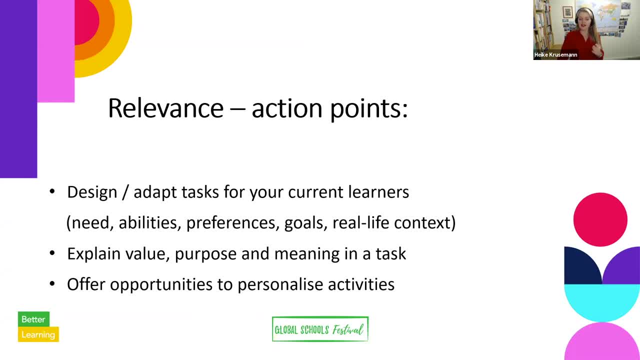 group when you're planning it in your head. So think about them like that And then in planning the next lesson, focus on a different subgroup or a different learner, And if you do it like that, then it will make your planning more specific and it will strengthen the link between the materials. 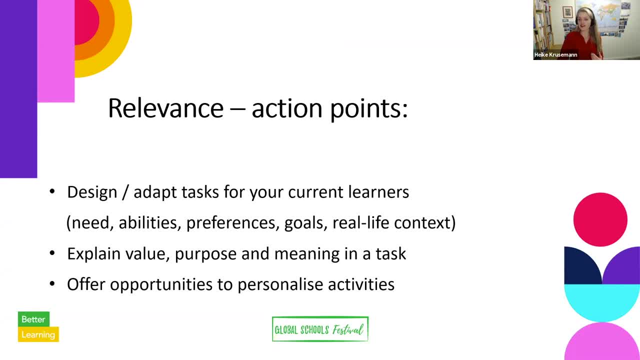 and between the learners, And some helpful questions to guide you in your lesson planning are: what do learners need to learn, What are their current abilities, What do they like to do? And, of course, offering a variety is always a good idea from an engagement point of view. 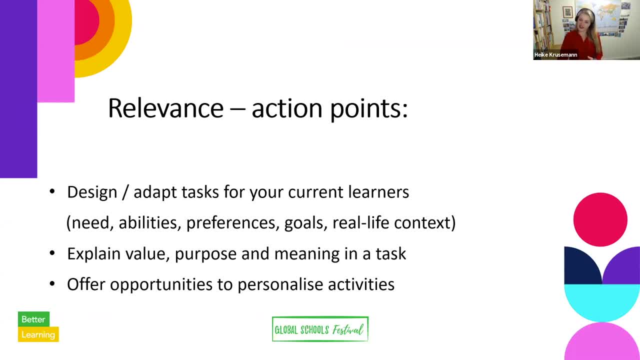 And what are their goals? Now, goals are different from what they need and what they like, because goals are all about learner beliefs And, last, what are learners' real lives like? And we always need to consider the social context of our learners and we need to be sensitive. 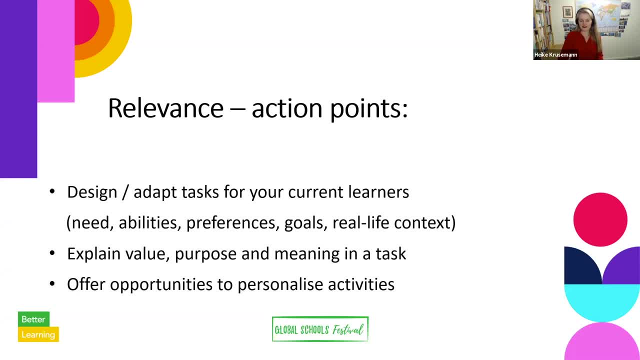 around how we use language and lesson content and be realistic in our outlook as well. Next is explain the value, purpose and meaning in a task, And we know from research that learners really need to see the value in a task in order to engage with it fully, So it's a good idea to make. 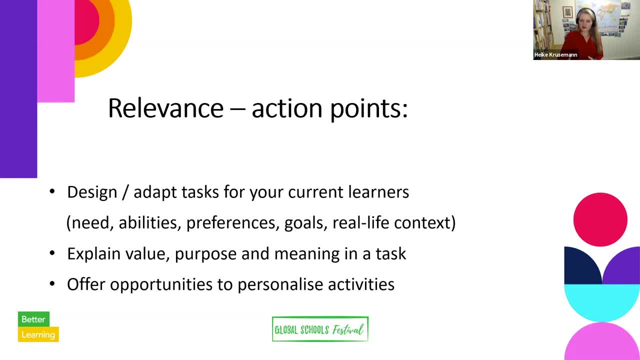 it explicit for them, or, better still, to get your students to work out what they think the value of the task is. So one of the things that I've always been very impressed with is the fact that this is a very, very powerful tool. Because I think that it's a very powerful tool. 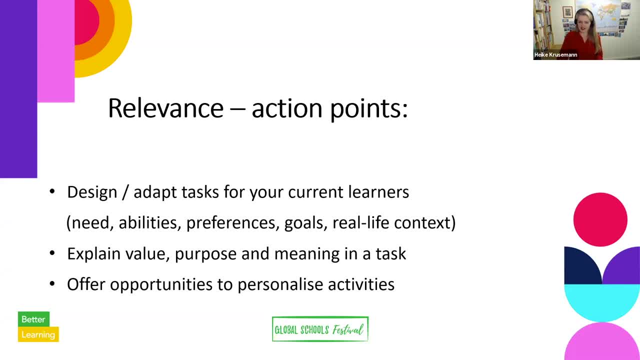 And if you've ever asked your students, or you've ever asked one of your students, or one of your students has asked you this question, you've said: why are you doing this? Have they ever said to you: why are we doing this? 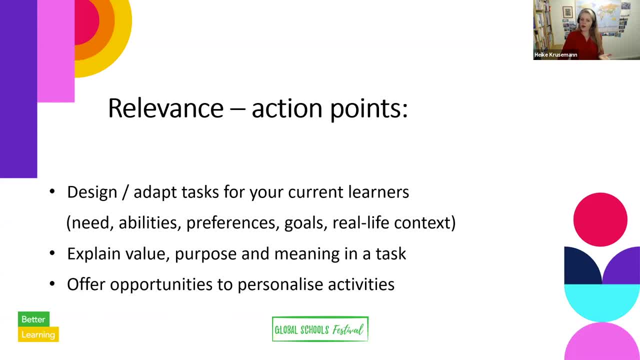 Type yes. if they've ever asked you that, Well, they've certainly asked me that, And so if you're saying no, then you're doing well, But there's again a lot of yeses coming up, So it's again a. 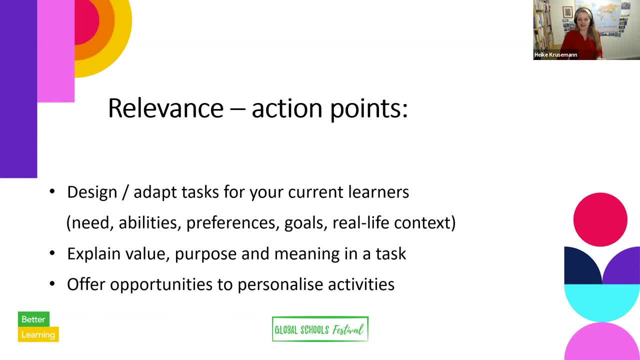 without you understanding the rationale for it is really not good enough, because for sustainable engagement, and certainly this is the case for older children and for adults, we need to go beyond the compliance phase. Okay, last is to offer opportunities to personalize activities wherever possible, and we already said that sharing appropriate personal details is a very bonding 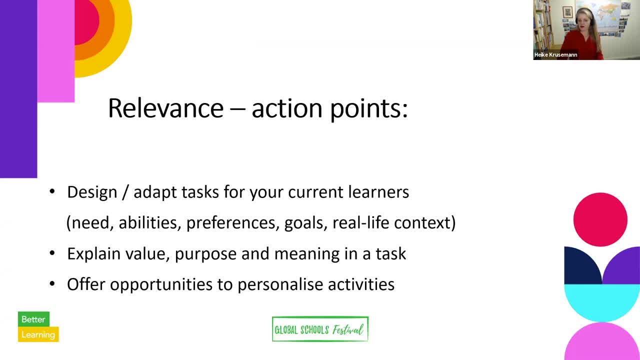 thing to do. So if you have a task about talking about other people, for example, then let learners choose who they want to talk about, for example, a famous person that they admire or someone they know that they admire. So I really like the British TV personality and chef Nadia Hussain. 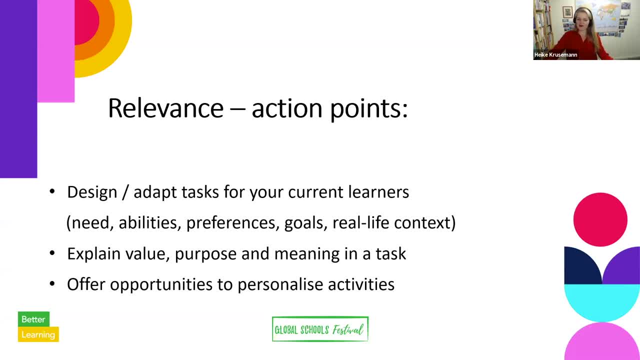 so I might start off by showing a picture of Nadia Hussain. So I'm going to use one of her cookbooks here with a picture on it, and I would model the expected outcome for my learners using a genuine person, Real life example that is authentic, and then learners can do the same and rather than 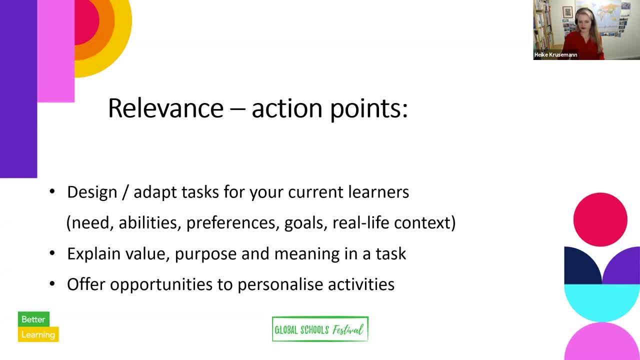 describe a generic photo or a stock image of a person from a textbook. Okay, right, so at the beginning of my talk I told you that I would be dropping in some small factual details about myself all through this talk, and so now I'm asking you: just type in the chat box what you have learned. 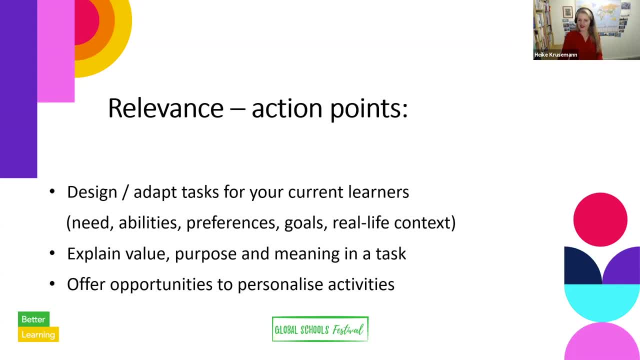 about me so far and I can tell you that there were five facts about me that I casually slipped into Into my talk. and people are. people are typing. yes, I like travel. yes, correct, I hate Mondays, not necessarily, just if, just in certain circumstances. yes, I live in the UK, like Nadia Hussain, like 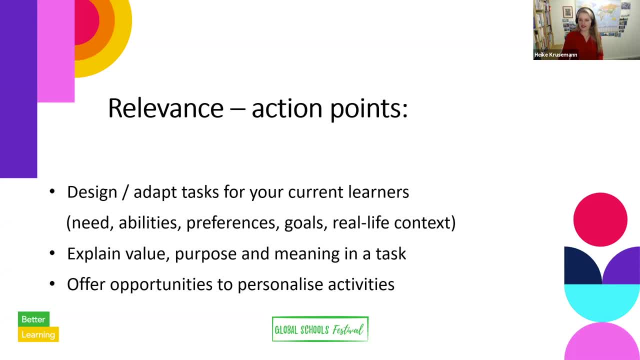 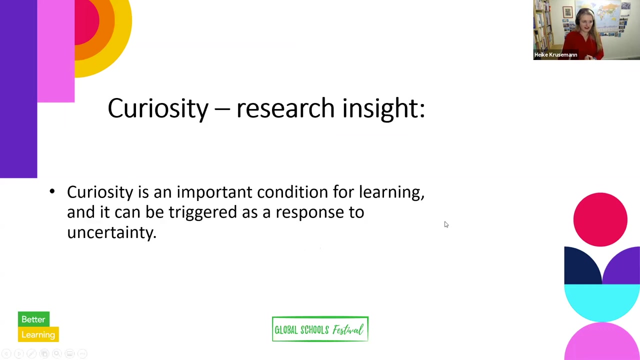 yes, very good, okay. so that that shows that you, you paid attention to these snippets of information that I dropped in during my talk, and so here's another question for you, though: would you have noticed or remembered any of this? No, I haven't noticed any of this, because I haven't told you to listen out for this, and my guess is you probably wouldn't, or maybe not as much. so what I did there is was that I activated your sense of curiosity, and we know from research that curiosity is an important condition for learning, and this can be triggered in response to uncertainty. so these little facts about me that would they would be new information for you, and also, importantly, you never knew when the next one would happen, so I'm going to ask you to tell us a little bit more about that. 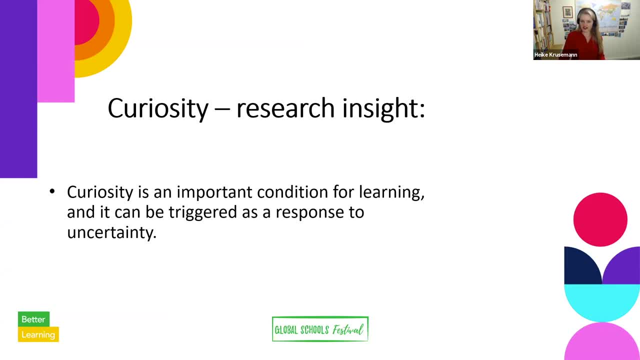 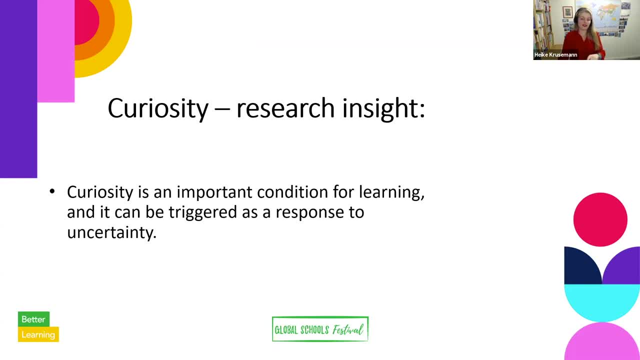 Okay, then they could write down the time of when you mentioned that or when something appeared. There are all sorts of possibilities for this kind of task or this kind of idea to work online or offline. So this was all about random rewards, but it's also much more satisfying for us to discover. 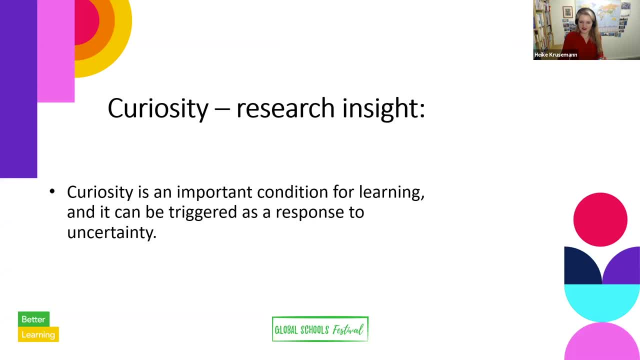 something for ourselves, rather than to be just presented with the information. So, for example, if you think of two presents that you might receive and one is wrapped and one is unwrapped, which one is the more exciting one? the wrapped one or the unwrapped one? 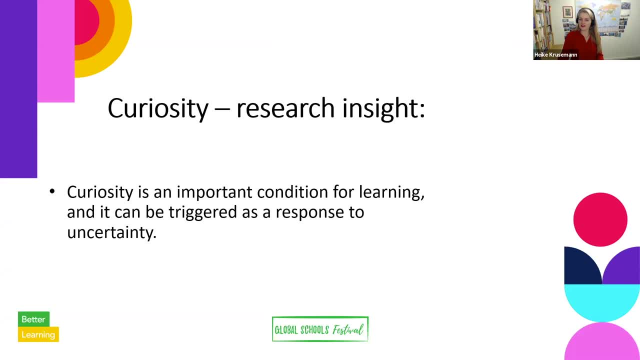 So, in the same way, letting learners to find out about things for themselves is much more engaging than just presenting them with the information, because there's always the danger they can just switch off, And you can use this for topic content, but also for working out the 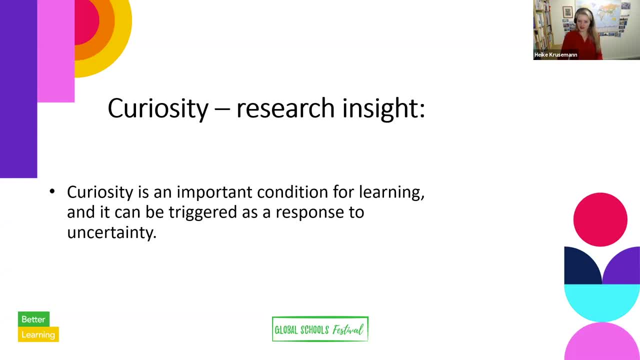 rules of language, And so the discovery, or the inductive approach for learning where learners work on the rules of language is much more engaging than just presenting them with the information. So this is a great example of how to work out something for themselves based on examples. 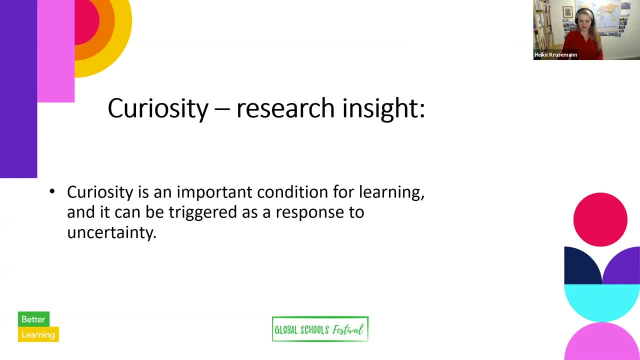 and scaffolded guidance is very popular for that reason. Second, we all have an inbuilt urge to find out how things work, and that's sometimes called the mental itch. So you can create a mental itch that your students will want to scratch. 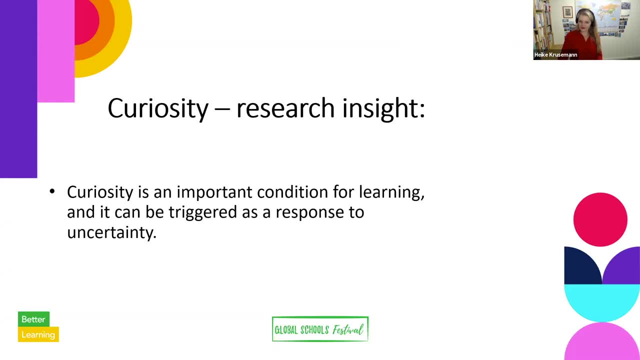 and you can do this by using elements of surprise or mystery, And we're all familiar with highly effective attention-grabbing strategies like cliffhangers in advertising in the media, in films and books. We know that this works, And so one way of using 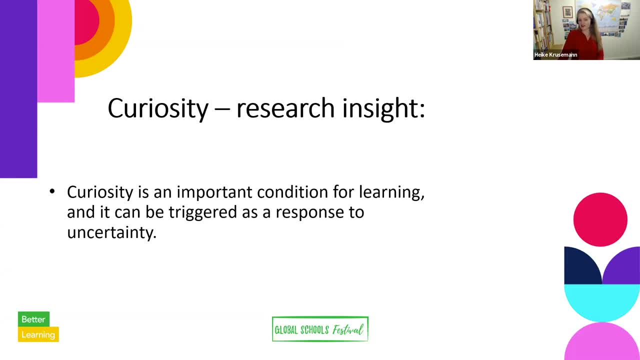 this in your teaching would be to end on a cliffhanger and get learners to speculate about what happened next. And this is related to the last point, which is use the power of stories. And again, as humans, we're all naturally attracted to a good story, not that we want to find out what. 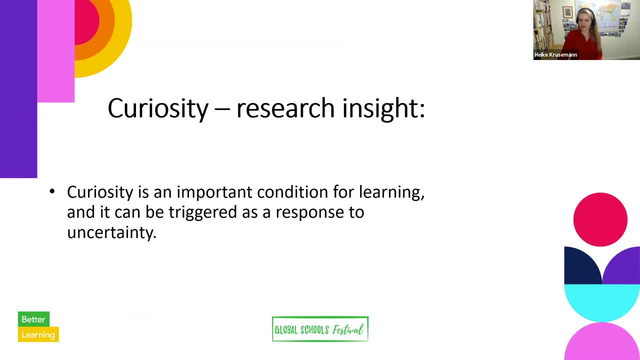 happens, but also that we remember information more effectively when it's structured in a narrative format, Because this is a format that's very familiar to us and we instinctively relate to it well. And stories appear not just to younger learners when they are used more commonly. 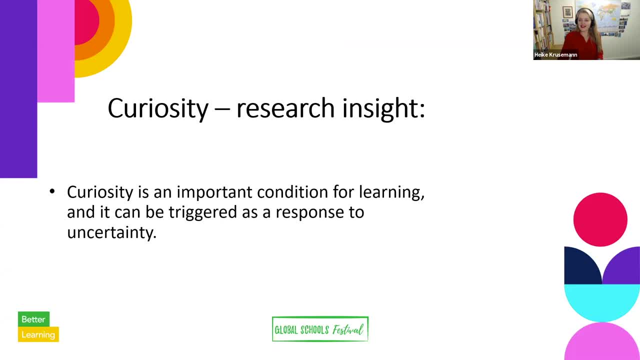 but really you can use them with learners of any age and I would like to encourage you to do that, And that's stories as input for teaching. but don't forget, we can also set creative tasks where learners are the storytellers, And that works with old school pen and paper, of course. 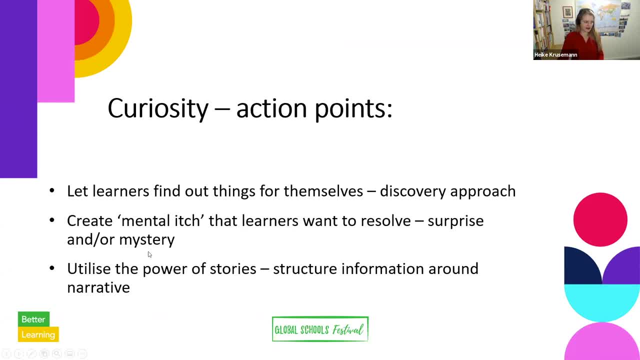 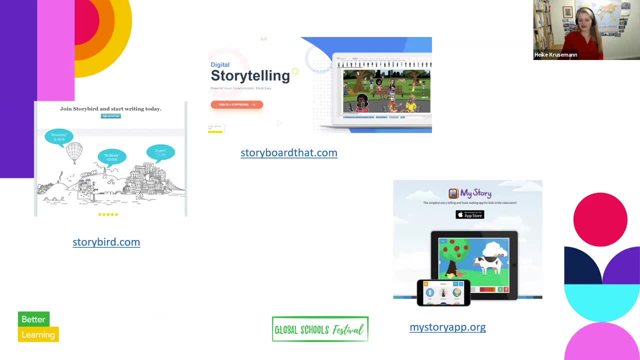 but there are also some really lovely digital tools as well, And here are a few on the board that I've brought up for you there. That's Storybird Storyboard, My Story, and I'm sure you know some others as well, And people are sharing some other. 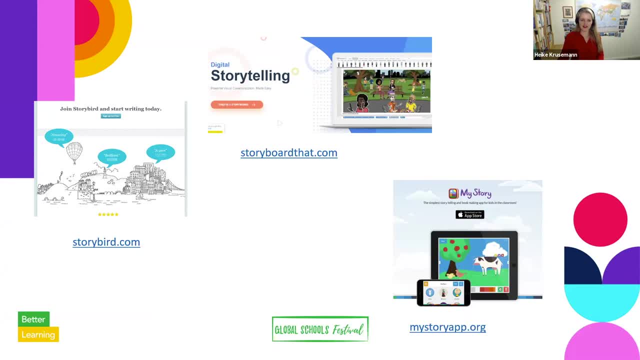 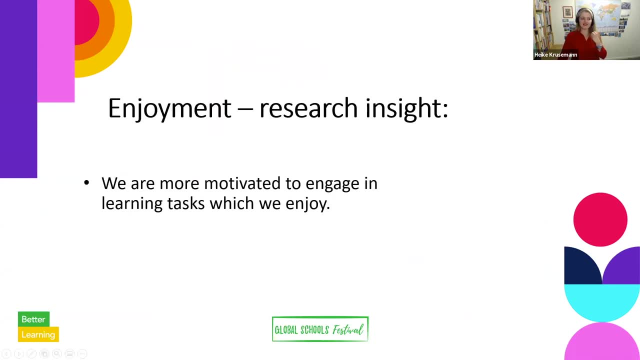 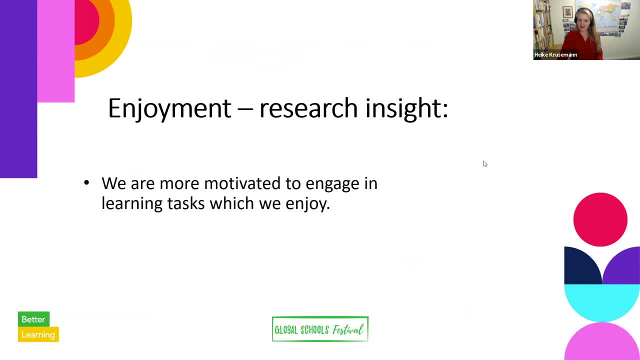 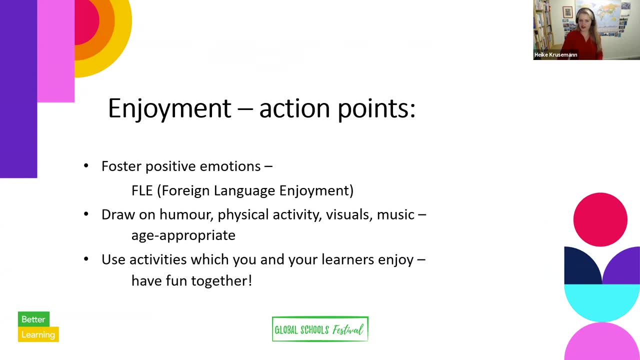 And that's why we're doing this And that's why we're doing this. So, especially in language teaching, do foster positive emotions, Do capture what is called FLE- foreign language enjoyment- because enjoyment is positively correlated with achievement And this means we enjoy what we're. 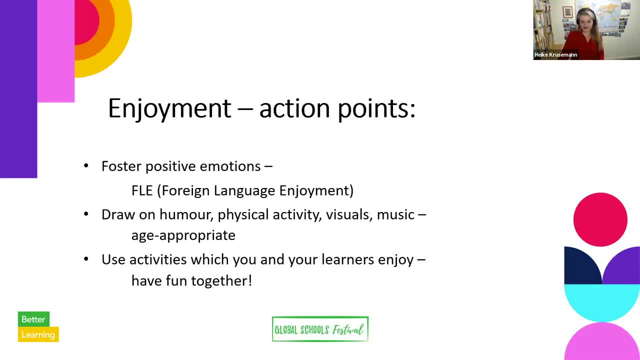 good at and we're good at what we enjoy, So this is a win-win. So do draw on humour, on getting learners active, on using visuals music. Again, you know your learners best so you can design tasks. 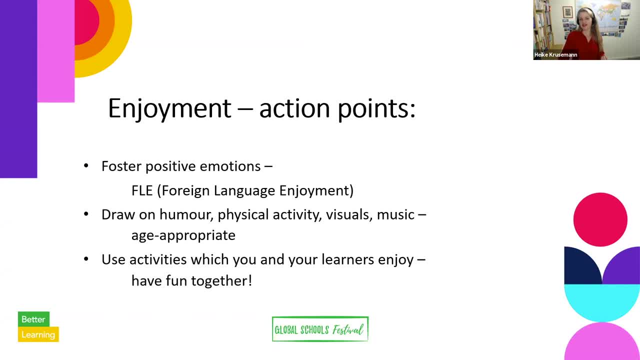 around what you both enjoy and what suits your context and the age group that you are teaching. Now, please don't be worried that if you're laughing with your class, that the message is that the lesson isn't serious or that it is not important. That's not the case at all, because we 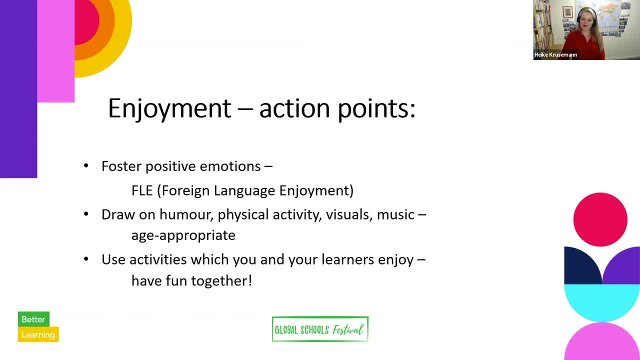 do take learning very, very seriously, But this doesn't mean that we have to take ourselves seriously, And this can be done in a very authentic and lighthearted way, For example, if something amusing has happened to you in your own life that may be appropriate to share with. 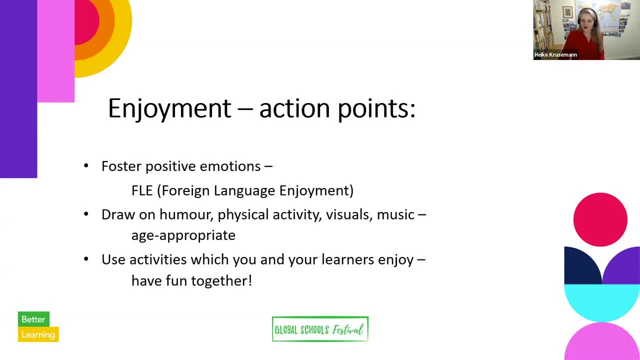 your students. then you could just try out doing that and see how that goes. And you could also ask students to share something funny with you in return. You could do that in the target language and everybody's happy. You could try out and see how that goes, And I wonder if anyone's ever 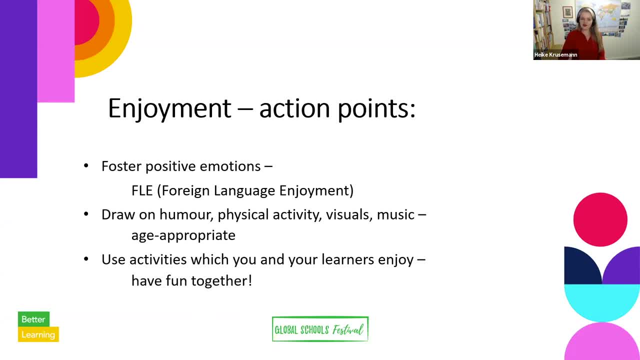 tried that. If so, just share it with us in the chat. So do use activities that you and your learners can enjoy together. Have some fun together. So your students seeing you enjoying teaching them and sharing a laugh with them. this will help a lot for them to connect with you on a human level, And it will again. 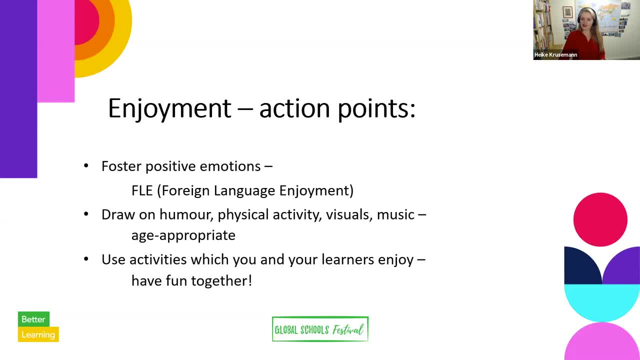 build social connections and trust And it's the social relatedness which we've seen at the beginning, which you all know, also as practicing teachers, is the underpinning of all successful learner engagement And from this stem the other building blocks of engagement which we talked. 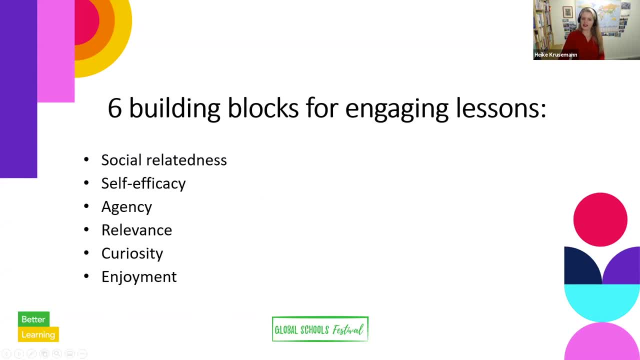 about, which are self-efficacy, agency relevance, curiosity and enjoyment, And if you address these building blocks in your teaching, then any activities based on them will be engaging for your students now and for the future. So hopefully, this talk will have given you some ideas for tasks that 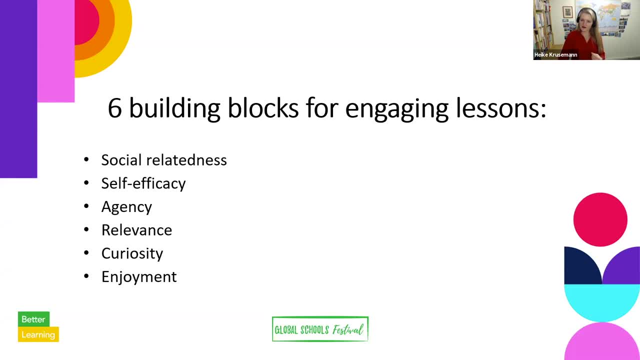 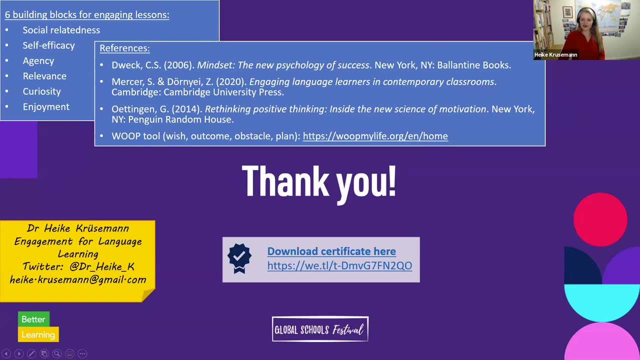 are engaging for learners, but, most importantly, also a sense of the bigger picture, of the foundations that these kinds of tasks are built on and why it matters. Thank you very much. Now you can download your certificate from this slide here, And I've also. 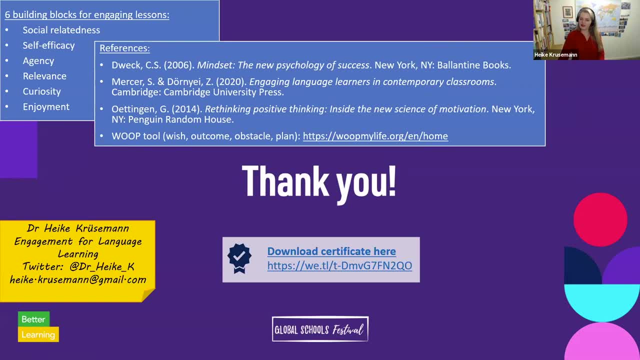 listed a reminder of the six building blocks of engagement, And also you can find here the reference list of the publications that I mentioned during the talk, And I believe we have a few minutes for questions. Thank you, Heike. We have about two minutes. 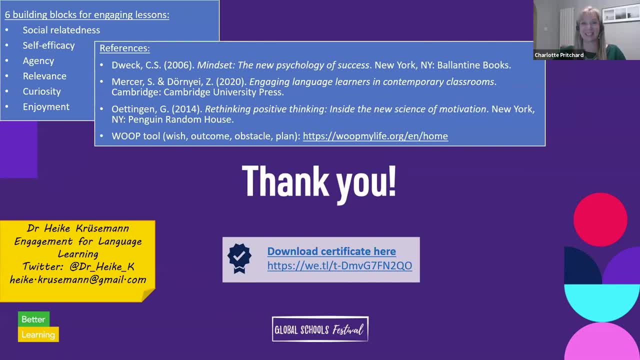 Oh, okay, But you're in such good flow, so we just Sorry, I got carried away, So I'm just going to throw one at you very, very quickly. We had a question from Facebook actually, which was about what can I do if I'm working on a topic and I really have no?